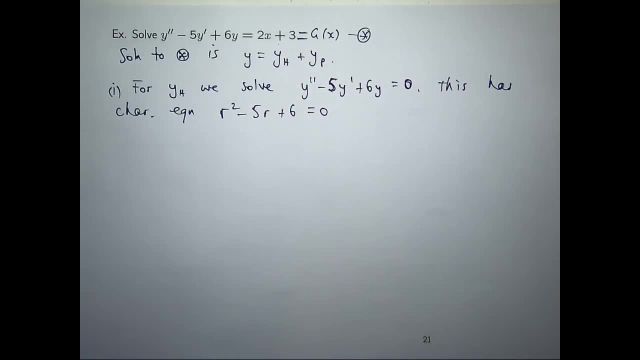 So what I can do is factorize that in this case and then look at the roots. So let's factorize this left-hand side. so my numbers are going to be something like minus 3 and minus 2 in my factorization. 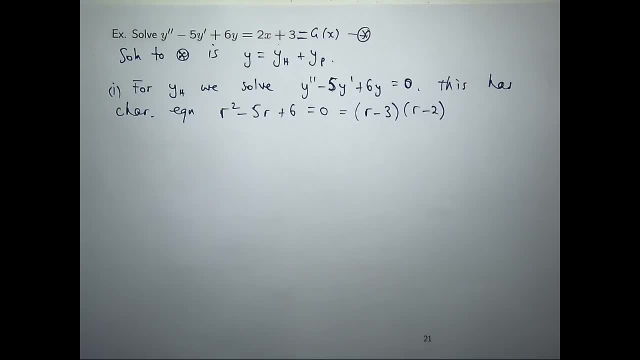 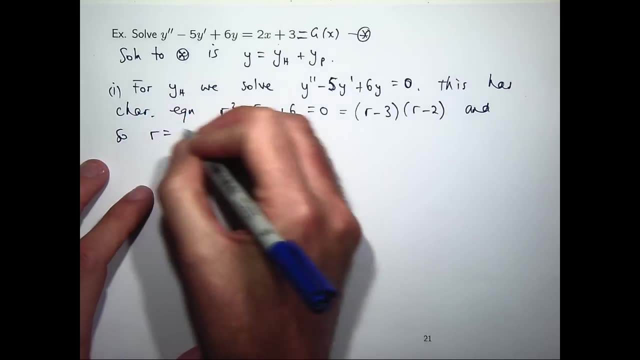 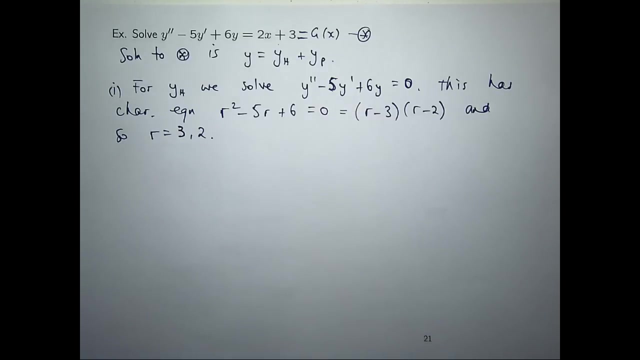 So the roots are going to be positive 3 and positive 2.. Okay, so we look at the roots. they are both real numbers And they're unequal. therefore, y sub h, the solution to the homogeneous problem will have a special form. 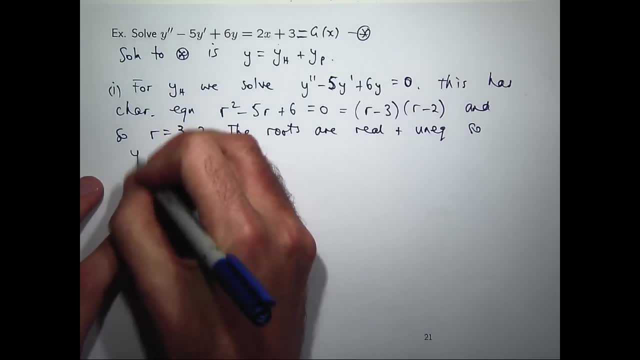 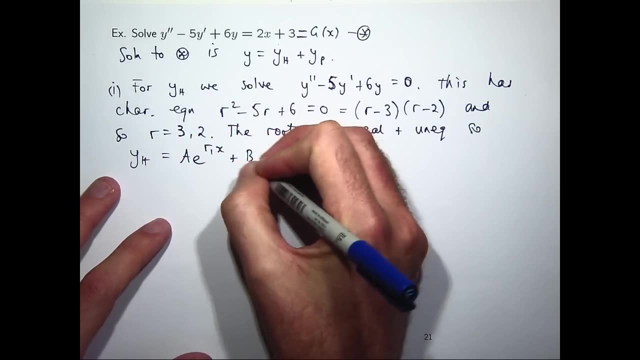 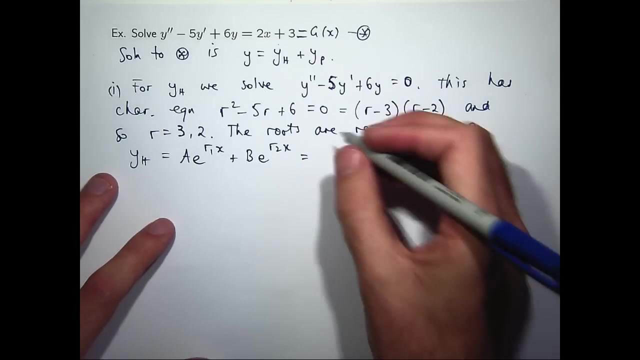 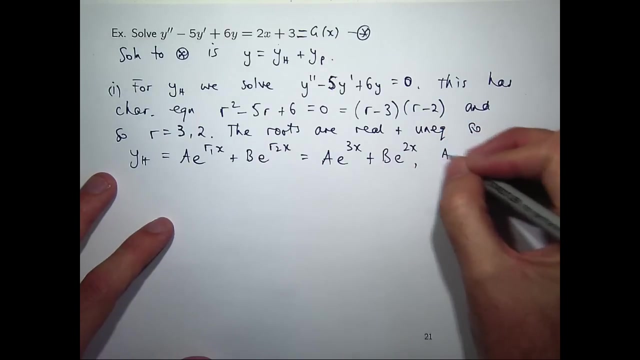 So the roots are real and unequal. so y sub h has the following form: Okay, r1 and r2 are just the roots, a and b are just constants. Okay, Now, it doesn't matter which way you put in the r1 and the r2.. 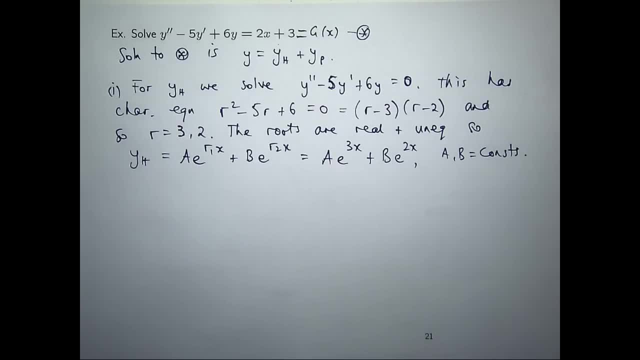 It's just general, a general solution. Okay, so that's pretty easy, right. As long as we can solve a quadratic and come and analyze the roots, we can come up with our homogeneous solution today. So this problem, Okay. the slightly more difficult part is constructing your y sub p. 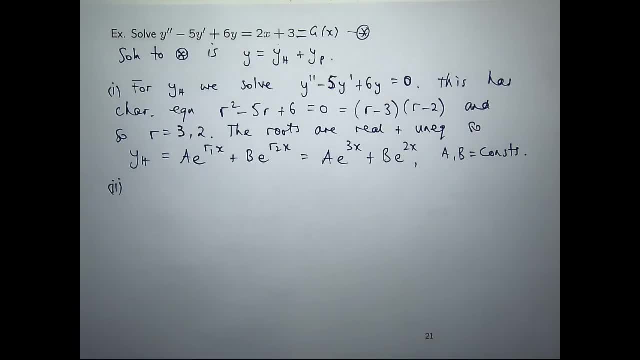 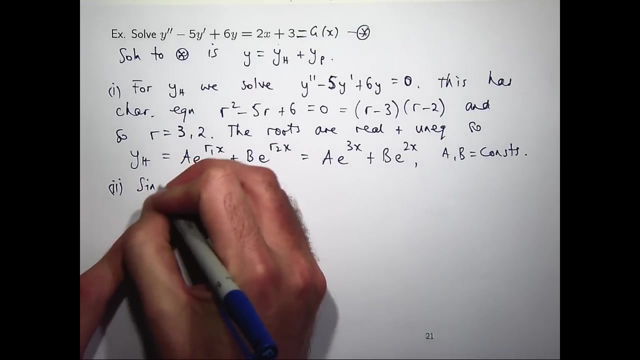 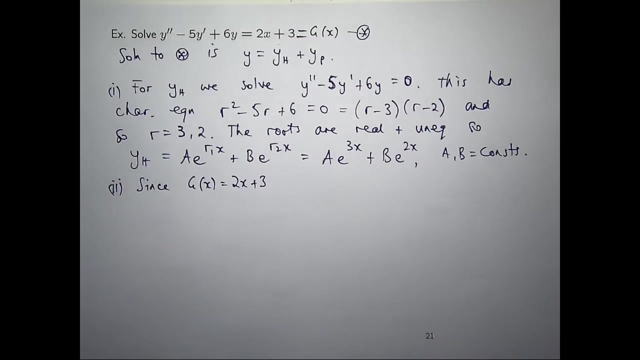 Okay, Now what we're going to do is look at the form of this g, of x, this right-hand side, and choose y sub p to be of a similar form. Okay, So let me show you. This is like a first-degree polynomial: 2x plus 3, just some sort of linear-type function. 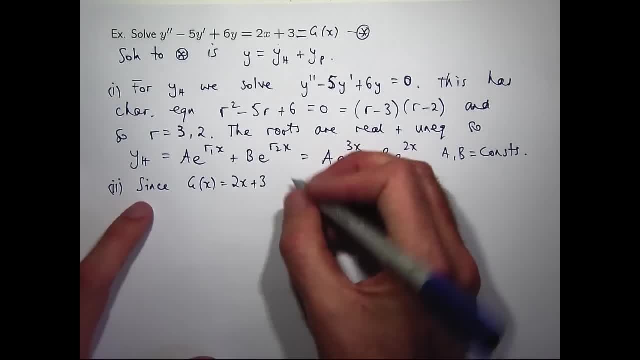 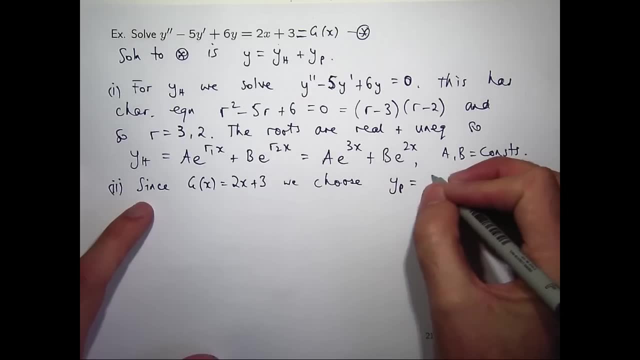 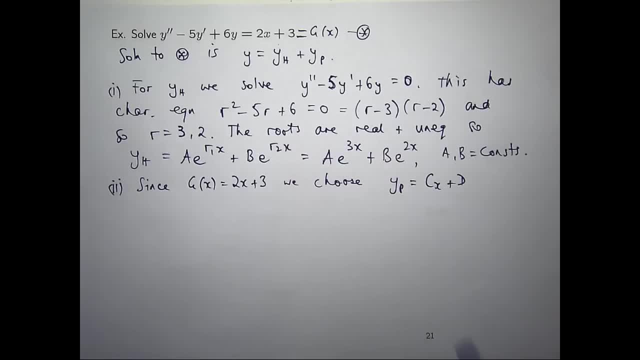 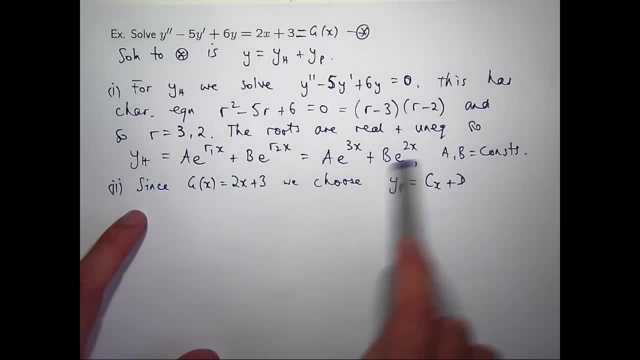 So what I'm going to do is I'm going to start with this and then I differentiate it once, differentiate it twice and sub into star, And then I'm going to equate the coefficients to find c and d. okay, I want to determine the constants, the coefficients c and d, in the bottom line. 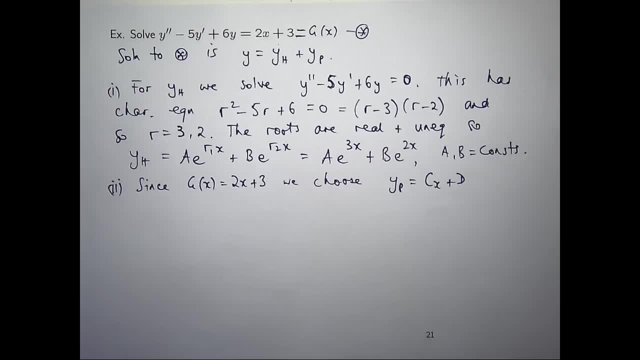 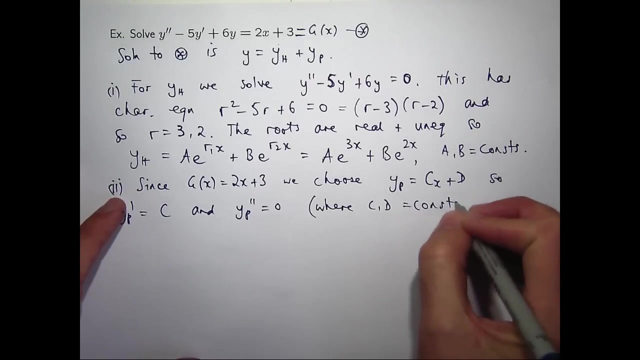 That's why it's called the method of undetermined coefficients, right? So if I differentiate- if I differentiate this, I'll get C, and if I differentiate again, I'll get 0.. Okay, so let's back substitute into the starred equation. 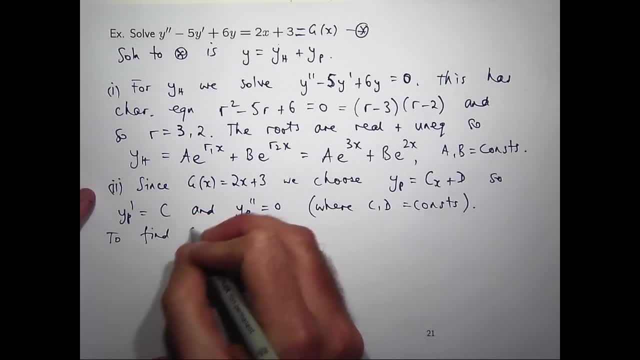 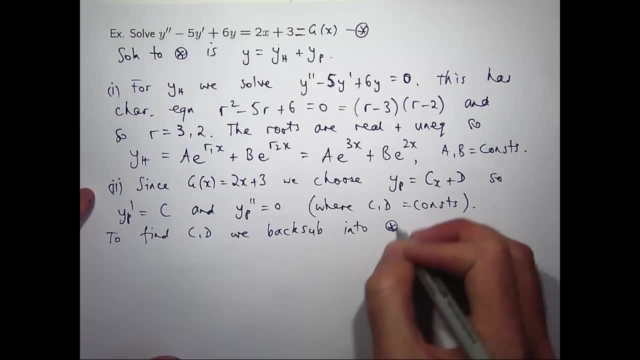 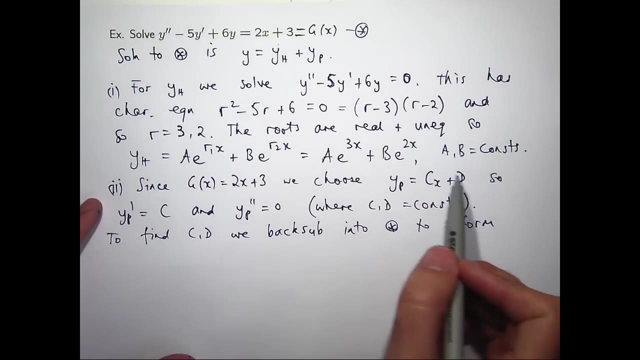 Okay, we're going to form the following: So, wherever we see y, we're going to replace it with Cx plus d. wherever we see y dash, we're going to replace it with C, and wherever we see y double dash, we're going to replace. 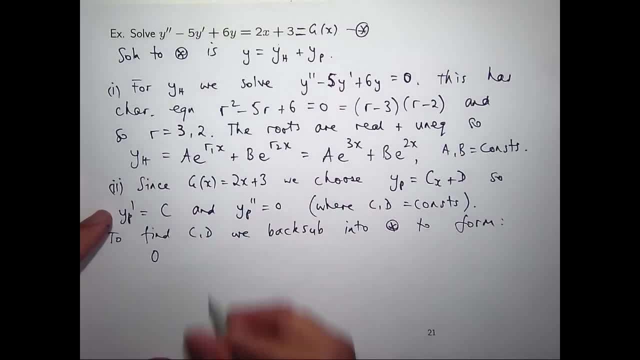 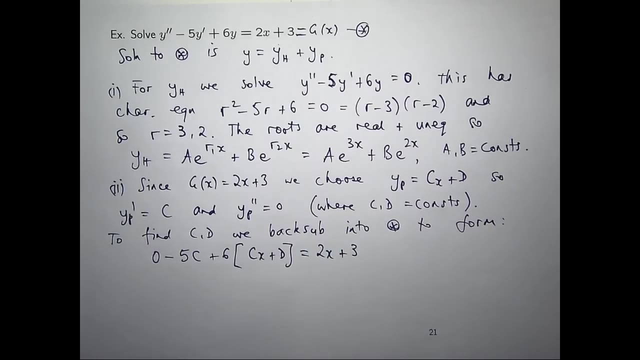 it with 0.. So star's going to become 0 minus 5x. 5c plus 6 times this equals 2x plus 3.. Okay, so all I need to do now is equate the coefficients. So what's C going to be? 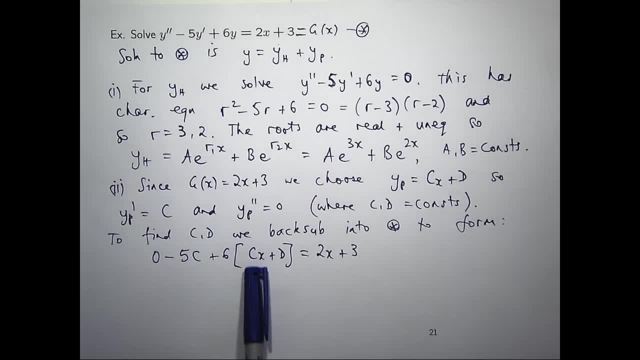 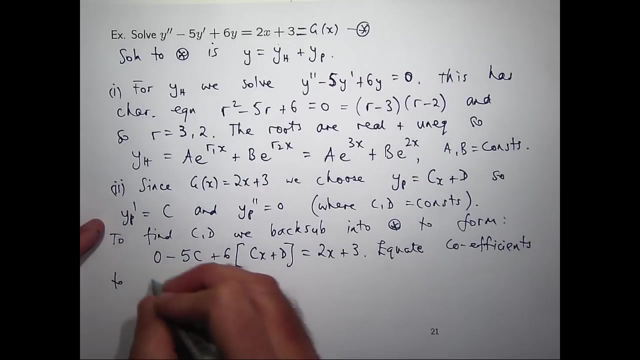 Well, we're going to. from the coefficients of x, we're going to get 6c equals 2, and if we equate the constants minus 5c plus 6d equals 3.. So we equate the coefficients to obtain the following: 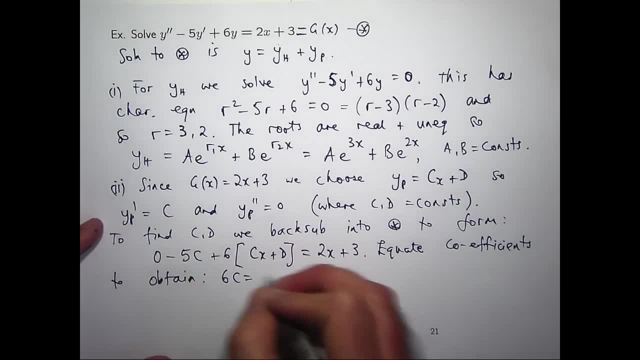 Okay, so we're going to get 6c equals 3, and minus 5c plus 6,. oh sorry, 6c equals 2.. Let me adjust that, Okay, And minus 5c plus 6d equals 3.. 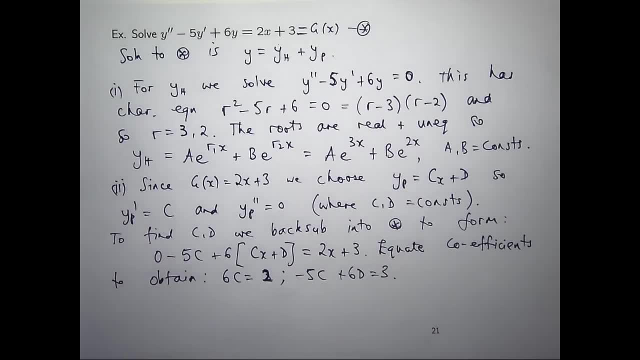 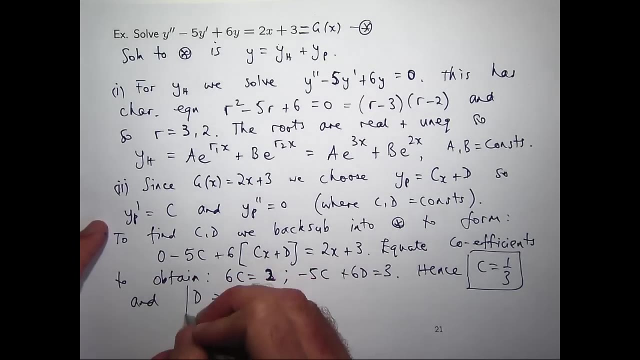 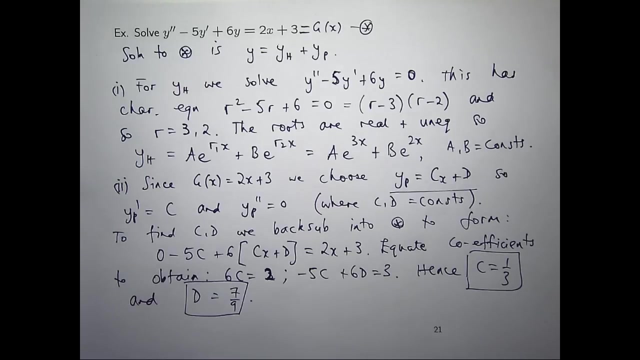 So we've got some basic equations there. Obviously, C's going to be something like a third and I can get d from the other one. Okay, d is 7 ninths according to my calculations. Okay, so now for this particular solution. we've constructed the c and d so that the 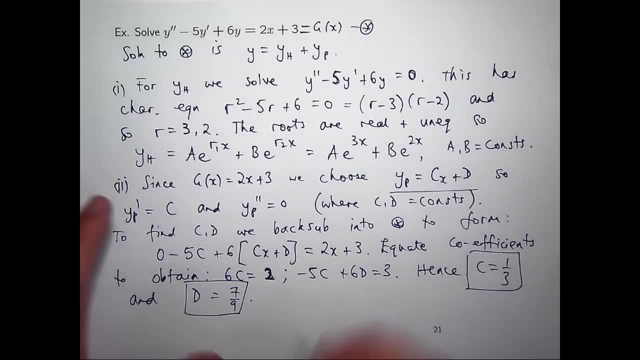 c is a third. That's the answer we're looking for And for this particular solution. well, it's a third, So we're going to compute the third. So there's our solution to some big problem, And 1. on the other hand, there's the bigger problem. We think it's going to be a third, and then we think it's going to be a fourth, So we're going to divide that by 4.. So we divide that by 4, and then we take that by 4, and we take it by 4.. 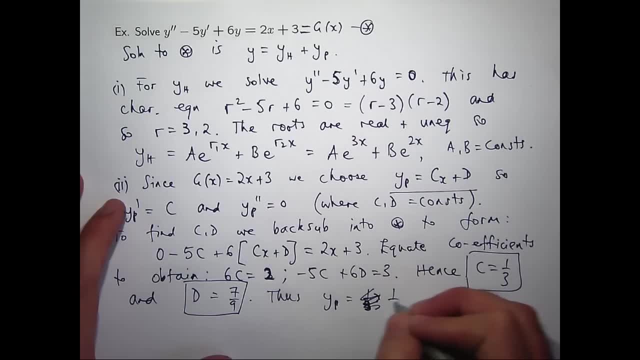 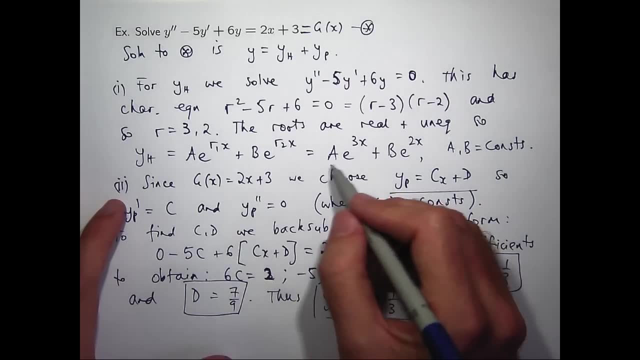 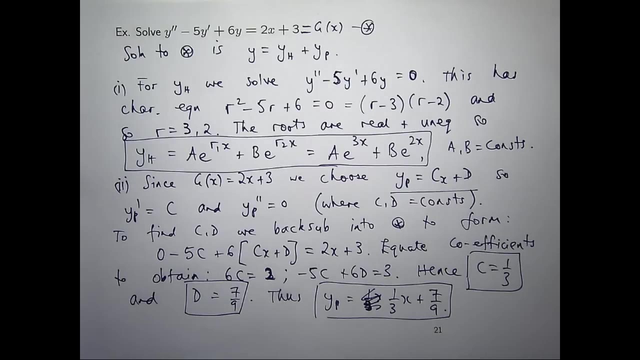 We have a third here and we divide that by 4. So that this will actually be a solution to star one third. Okay, so there's my particular solution. There's my solution to the homogeneous problem. What we do is we take those 2 and we add them together to form the general solution, that's. 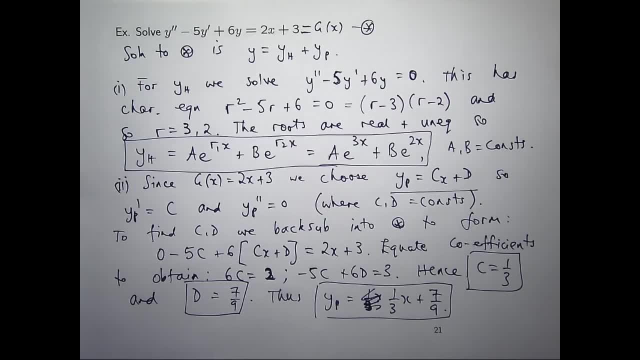 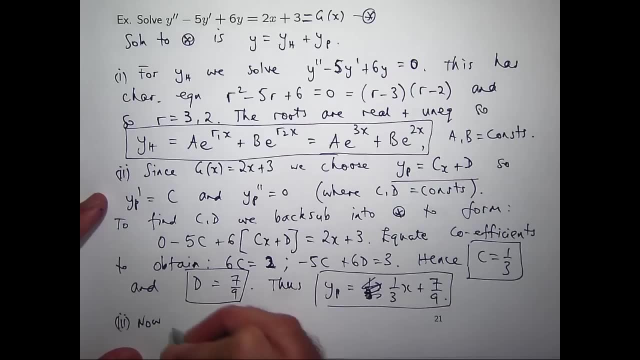 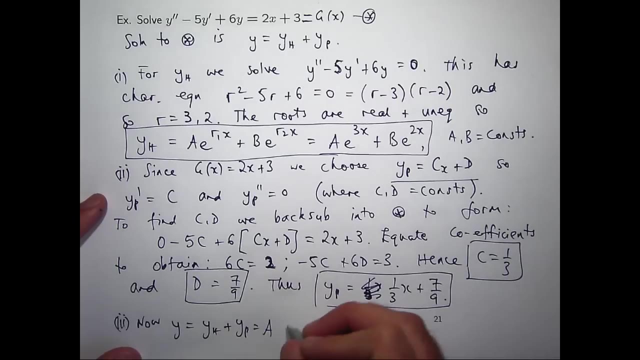 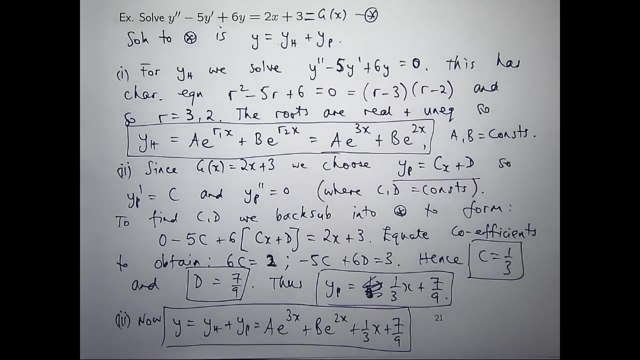 going to be a third to my original ODE star. so you feel like this is like a third step, okay. so it's this, okay. now, when you're doing the um- you know doing these kinds of questions- of course you don't have to put all this detail in, but I've just put it in to explain it as I, as I solve it. 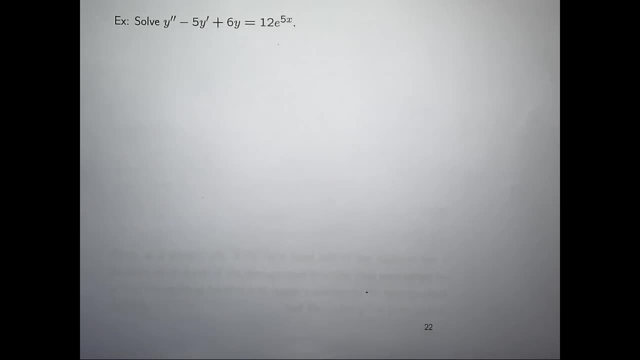 all right, here's another one where the right hand side is not a polynomial, but it's a exponential function. so how do we handle that case? well, I'll do this one a lot quicker, because if you look carefully, the home, the home, the resulting homogeneous problem: the left hand side equals zero. 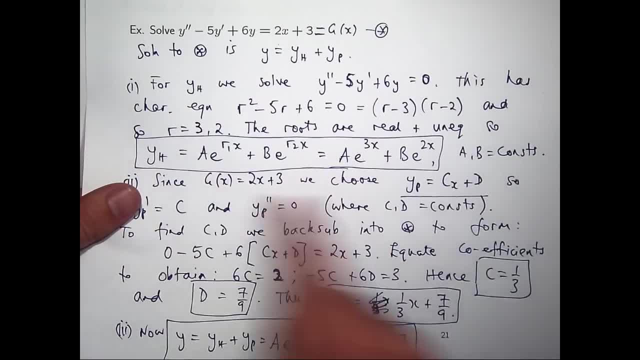 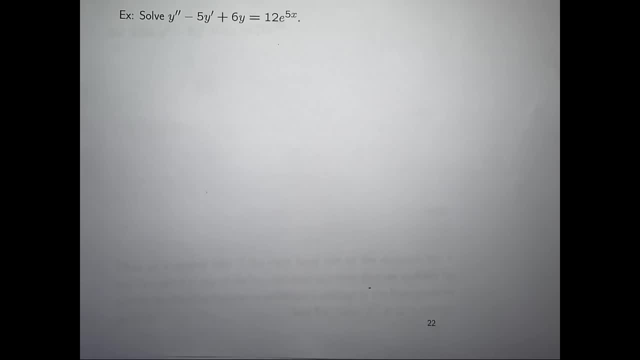 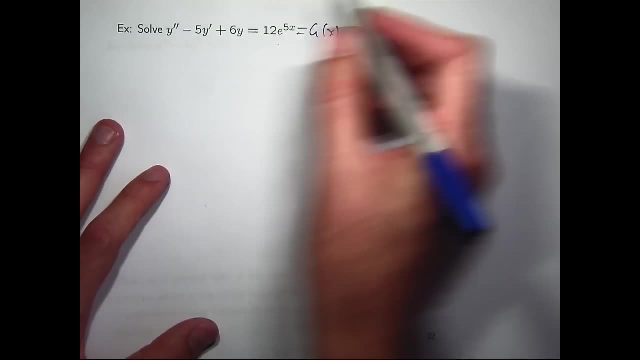 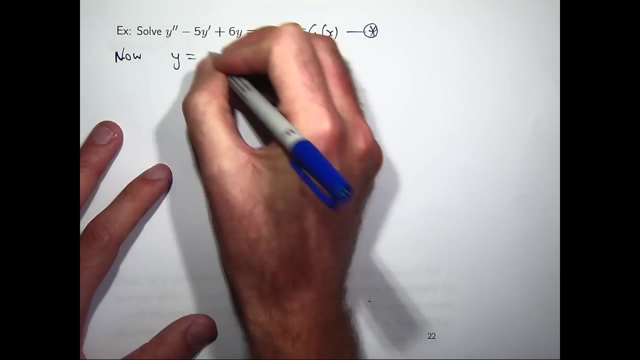 is the same, so I don't have to for this problem. I don't have to go back and do all this stuff again, okay, okay. so here the form of my right hand side has changed to an exponential function, so let's call that star from the previous. 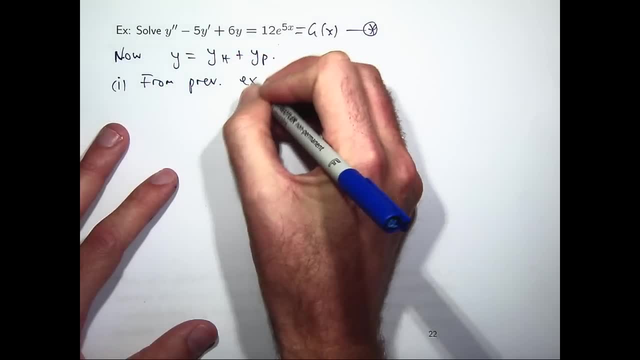 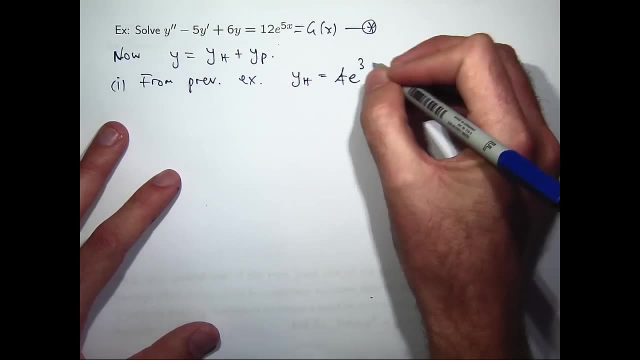 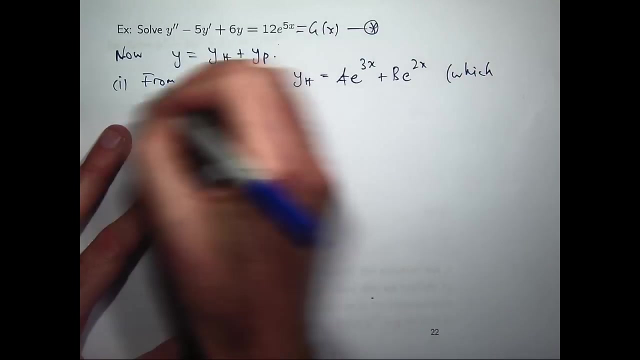 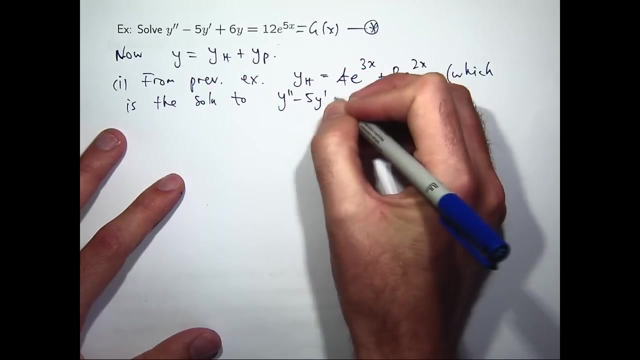 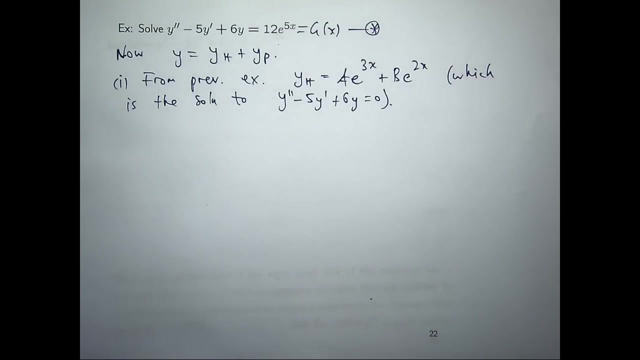 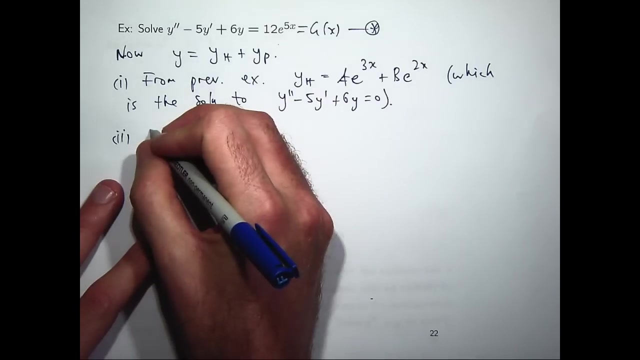 example, y sub h is just the following: okay, so I don't really have to worry about um writing that out here. big a and big b are constants, arbitrary constants. so how do we construct a particular solution? okay, okay, so we look at the form of g of x. it's an exponential function. 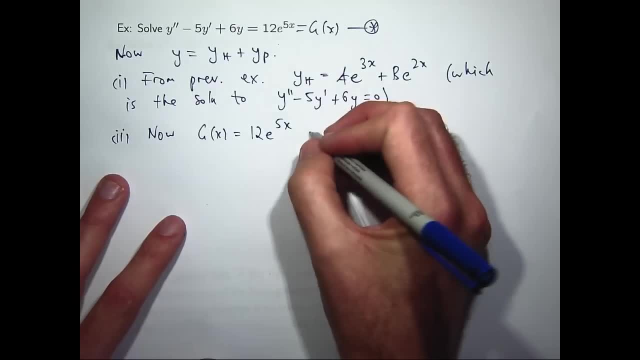 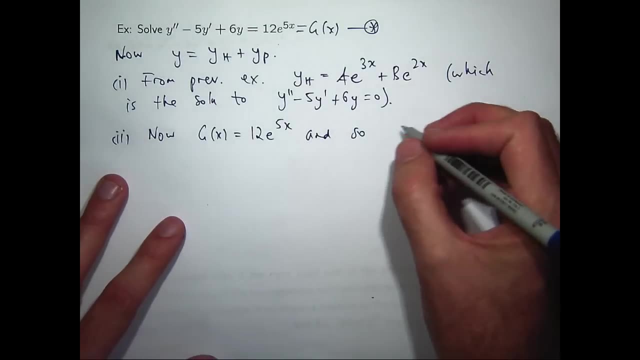 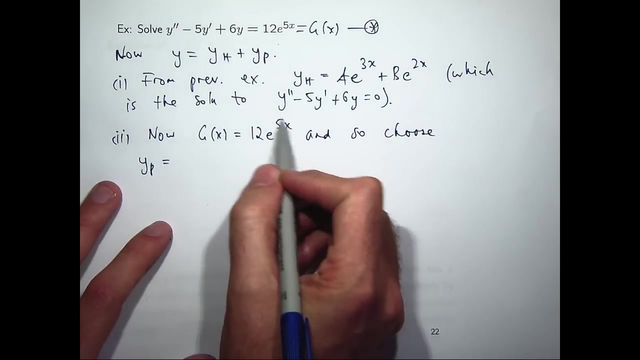 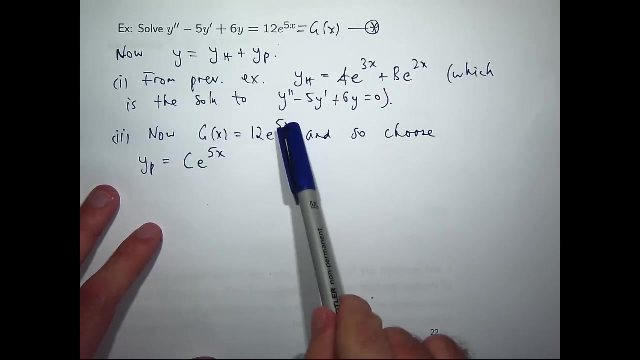 and what I'm going to do is use that to construct the form of my y sub p, my particular solution. okay, so I'm going to keep the five x, but just have a constant times e to the 5x. okay, So you want to keep the 5x? 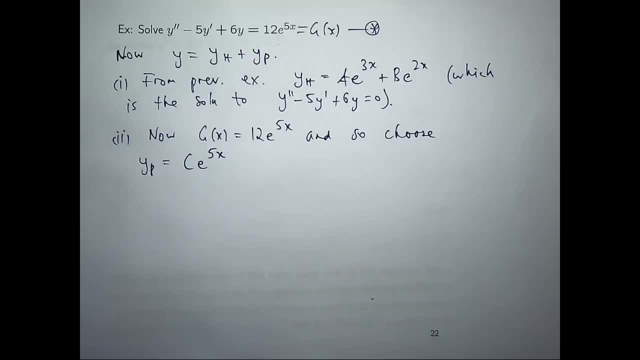 but just have an arbitrary constant at the front. Okay, so what I would like to do in this second step is determine the value of c such that this particular constructed solution will satisfy the original equation. okay, Okay, so let's just differentiate once. 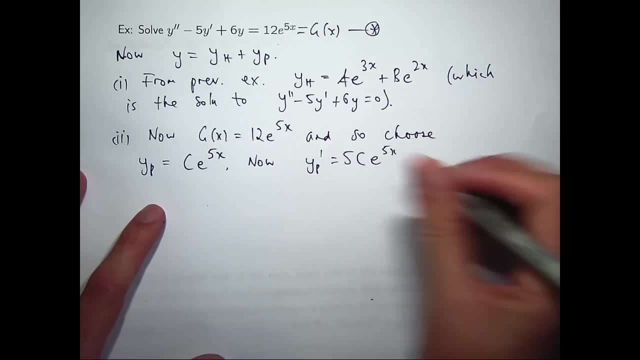 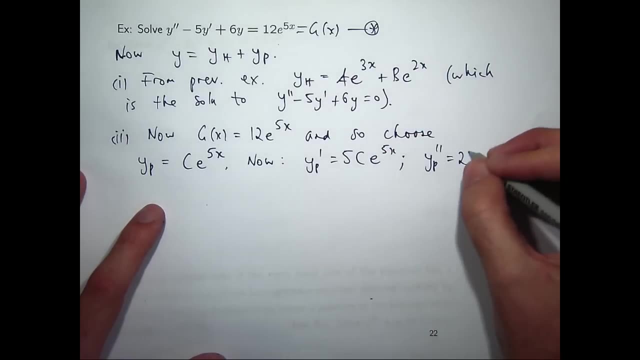 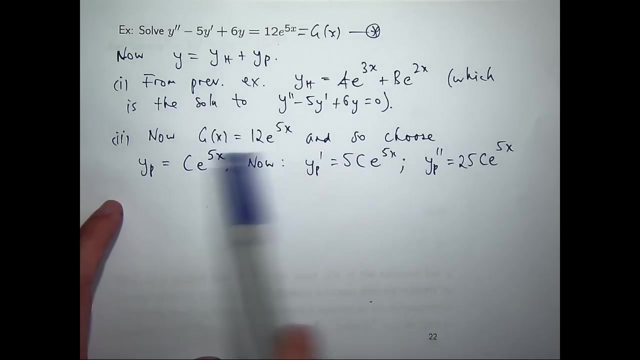 I'll get 5c e to the 5x. Differentiate twice, I'll get 25, so that 5 comes to the front again. 25 c e to the 5x, And what I'm going to do is sub in these three functions into star. 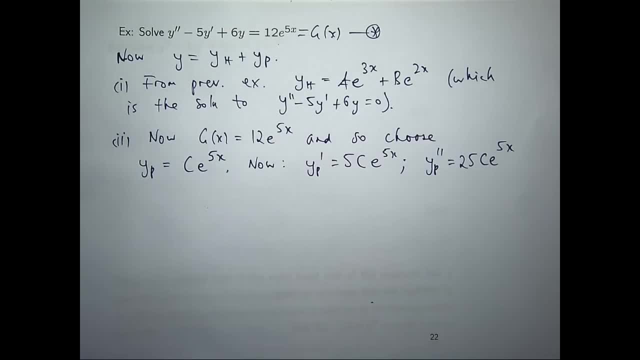 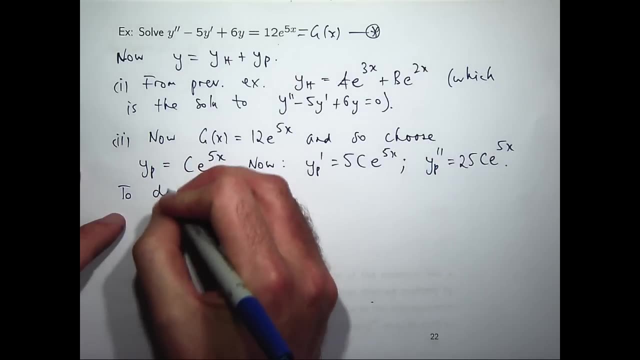 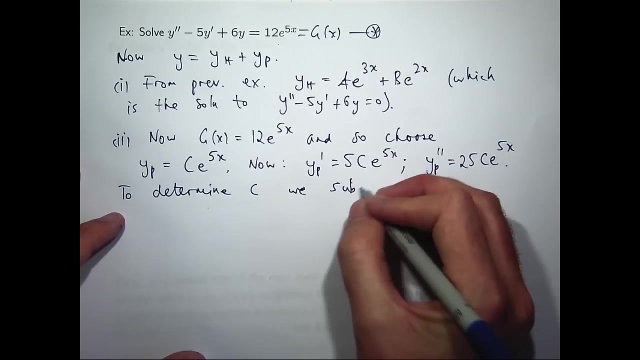 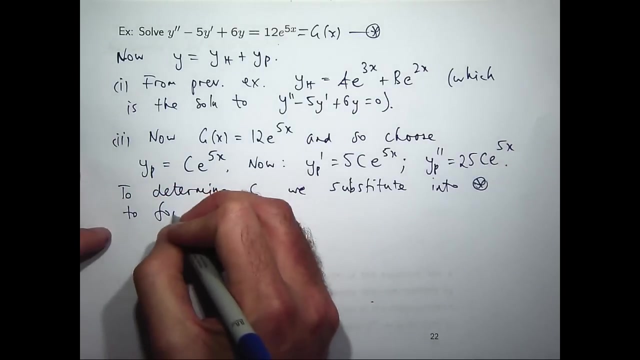 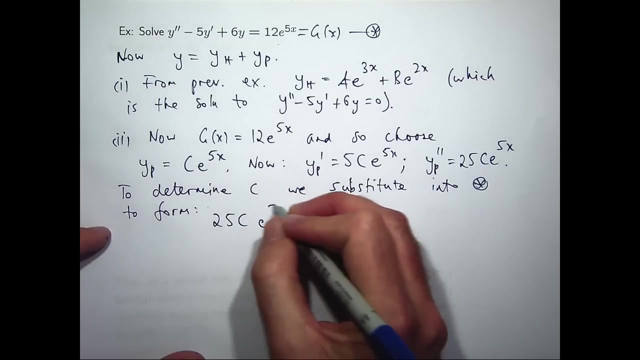 and then I'm going to equate the coefficients and find the value of c. that makes this a solution. We substitute into star to form the following: Okay, so y, double prime. we replace that with this: 25 c e to the 5x minus 5y prime. 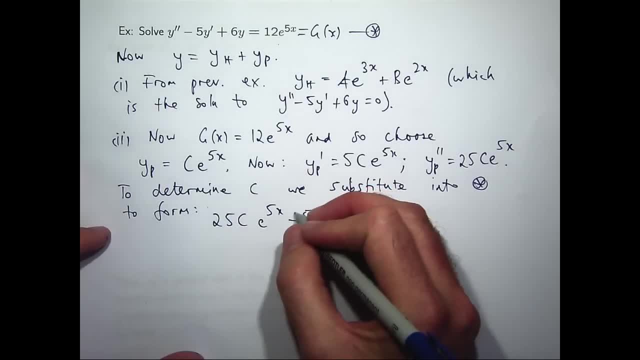 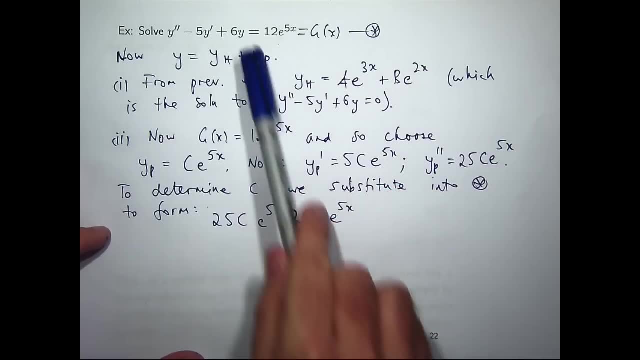 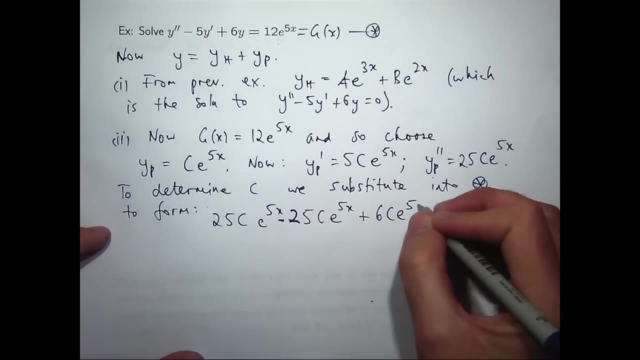 Well, it's just minus 5 times that, Oops, so that'll be a minus 25.. And plus 6y. so we're going to get the following: And the right-hand side is just 12: e to the 5x. 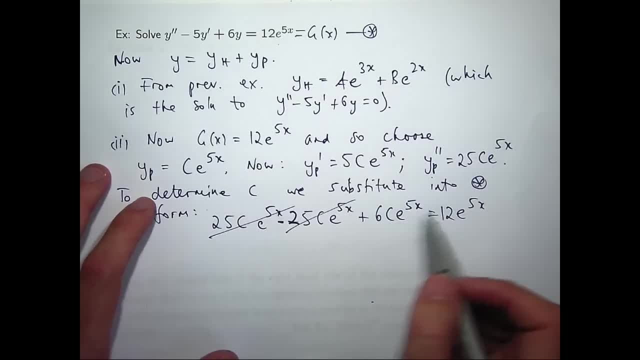 So you can see these first two terms are going to cancel off and I get the following. So, again, if I equate the coefficients, big C is going to be something like positive 2, right, What's that? Not something like positive 2.. 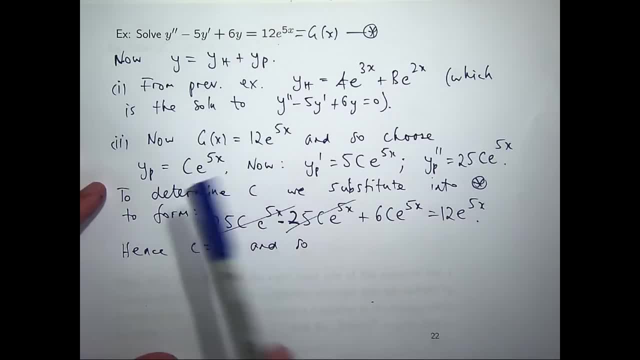 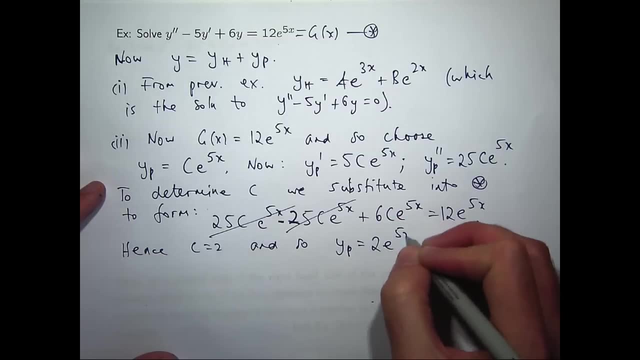 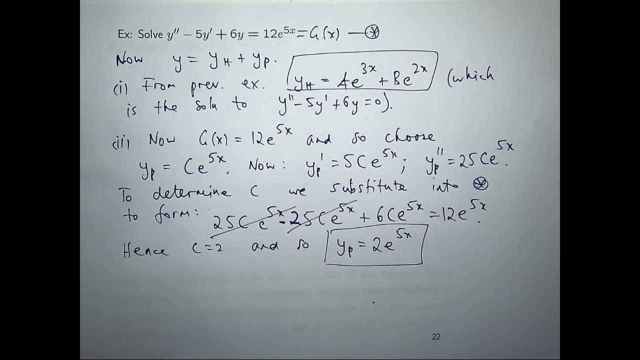 Hence, big C equals 2.. And so what's our c here? It's 2, so I'm going to get 2 e to the 5x. So we've got our homogeneous part, We've got our particular solution. 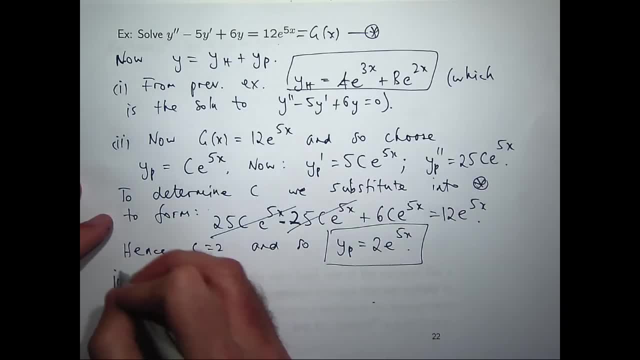 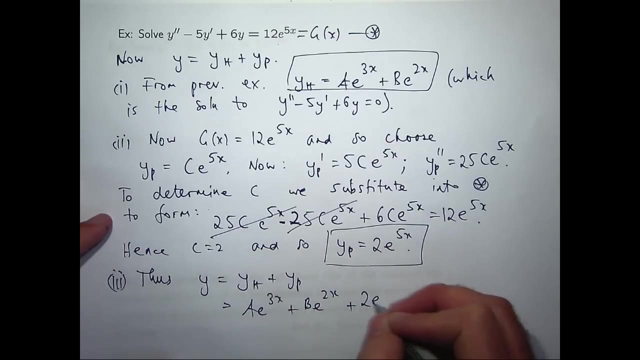 so let's just add them together. So I'm going to get something like a- e to the 3x plus b, e to the 2x plus 2, e to the 5x, where a and big A and big B are constants, arbitrary constants. 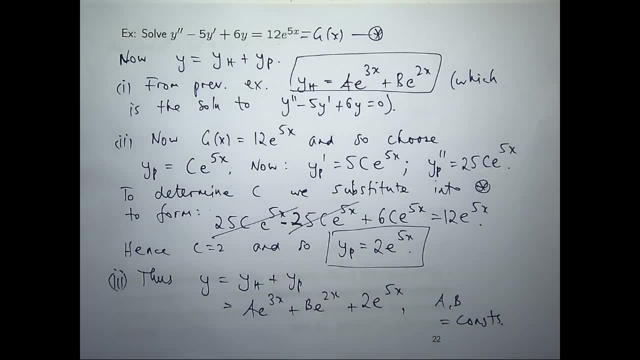 Now, can we determine big A and big B? We could determine that constant big C in there, but can we determine big A and big B? No, Why not No initial conditions? Yeah, we don't have enough information If we had some initial conditions. 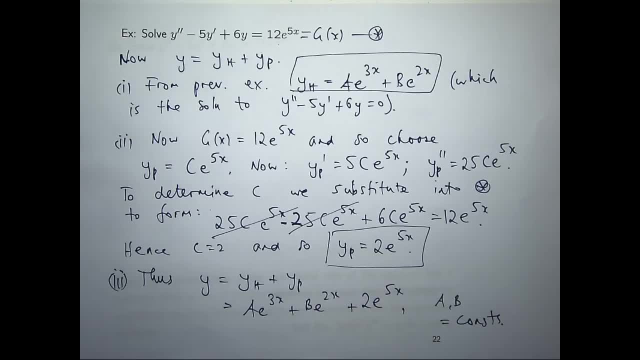 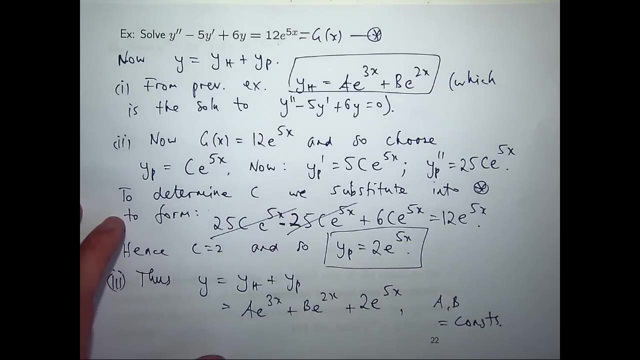 some extra information coupled with star, then we could go back and, you know, use this to determine big A and big B. Okay, So let's say you got down to this part and you know you couldn't balance these things by choosing a value. 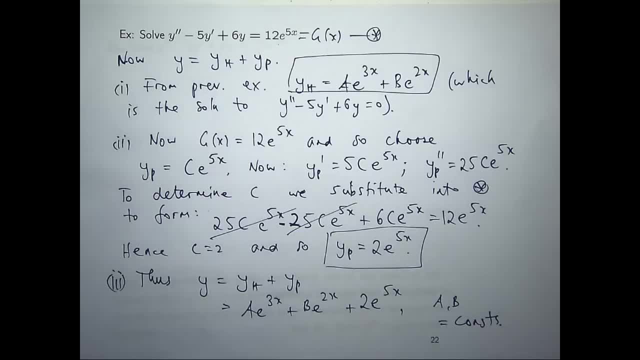 of c. okay, Sometimes you'll get down there and you're going to get something like this And you just can't solve. you can't solve, you can't find a value of c that'll satisfy that the thing. What does this mean? 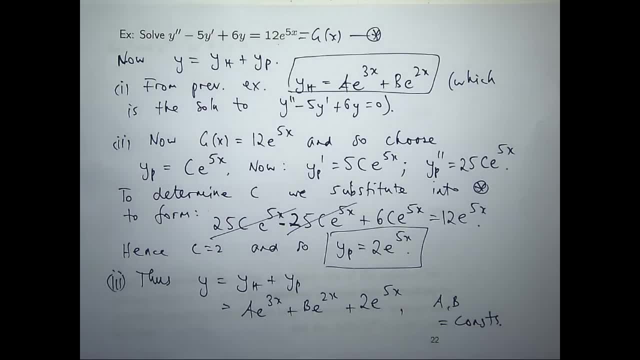 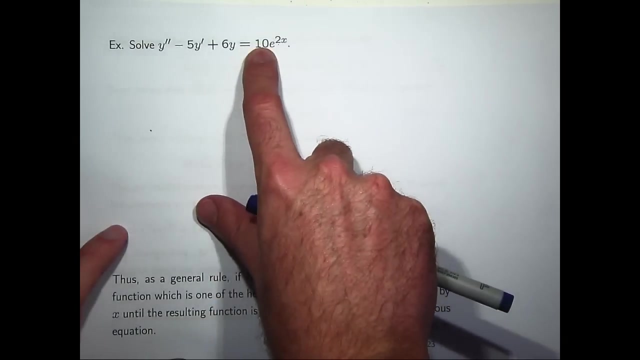 Well, it means either you've made an incorrect construction, starting with your y sub p, or you've differentiated wrongly. Okay, Any other questions so far? Okay, Now in your. I think you've got a question. I think you've got a 12 here. 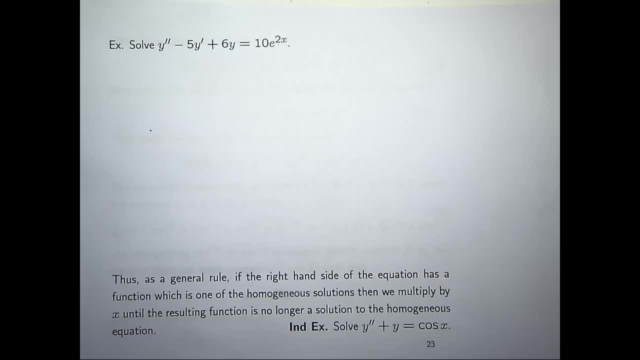 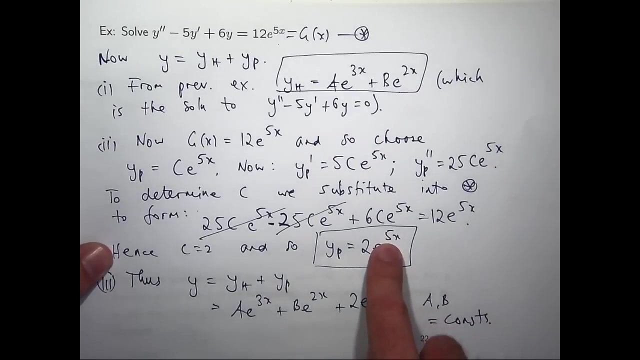 I've got a 10. So make sure you change that. Now. this is a good question To compare it with what we've done before. let me just put this back for a second. What happens? right, you can see when I add this solution. 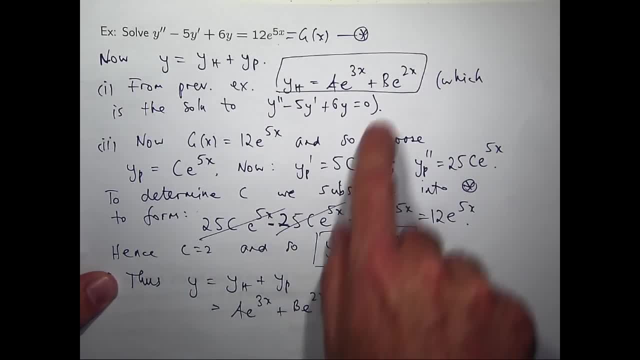 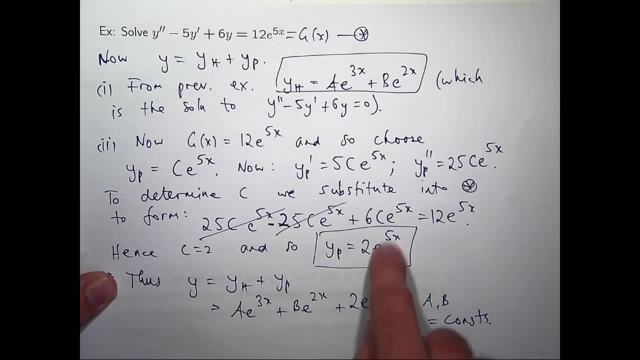 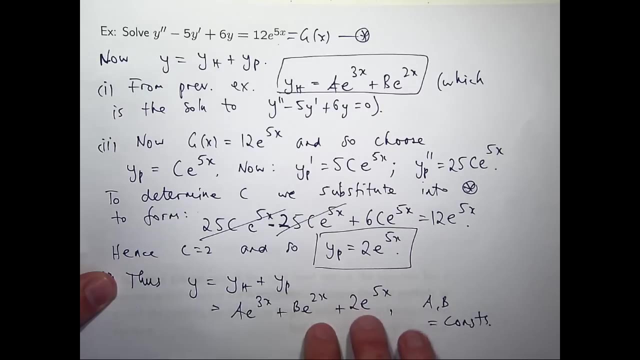 with this solution to form the general solution. each this is adding something new to this. okay, If this was an e to the 2x or an e to the 3x, it's already contained in this homogeneous solution, So if I was to add them together, 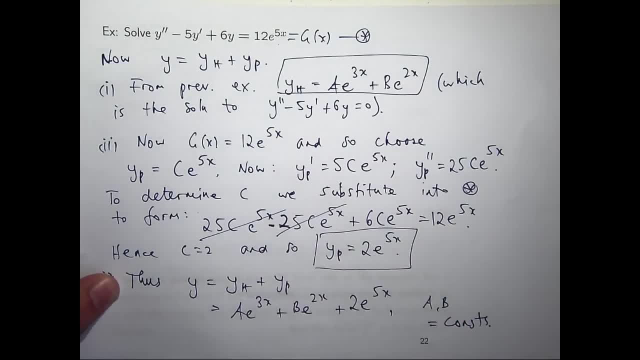 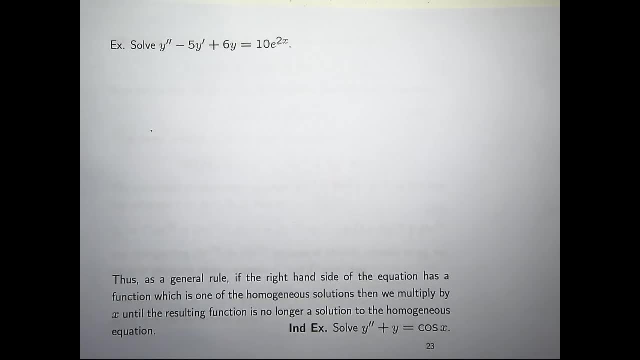 this part wouldn't be adding anything new. It wouldn't be bringing anything new to the table. This is something you need to be conscious of and, in fact, it's covered in this particular example, So this is a very good example. 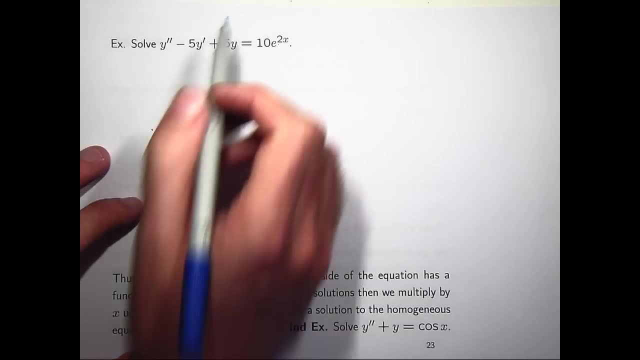 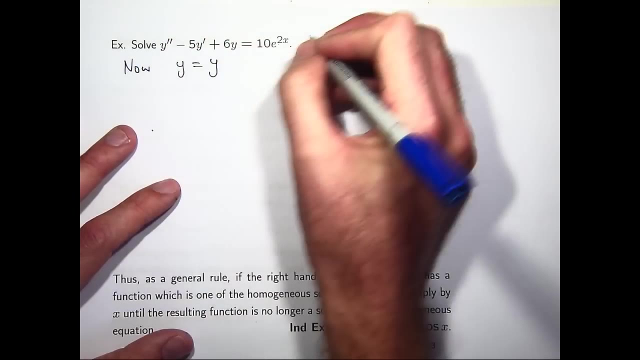 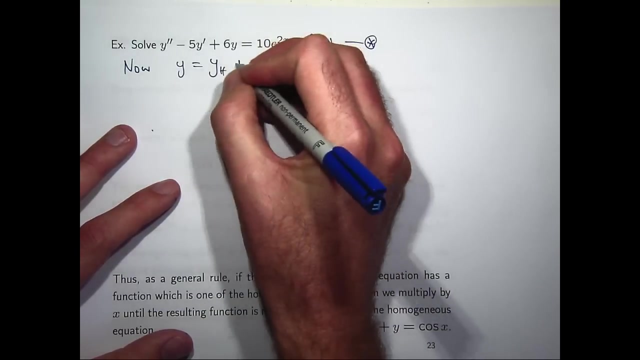 Okay, Again the homogeneous solution. it's very easy to calculate because we can just take it from the previous example. So here we've got a right-hand side. that is again an exponential function, but, as we'll see, a little bit of care needs to be taken here. 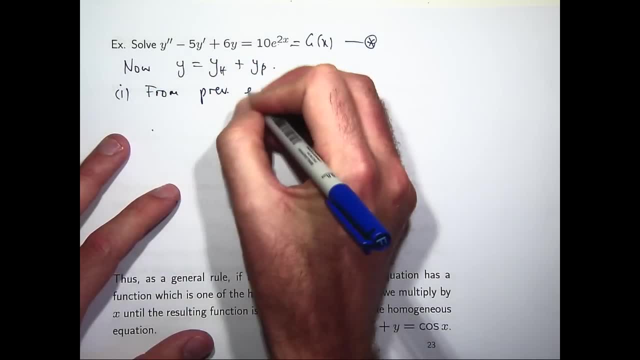 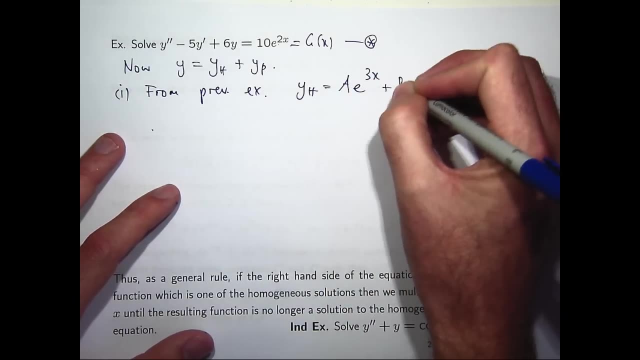 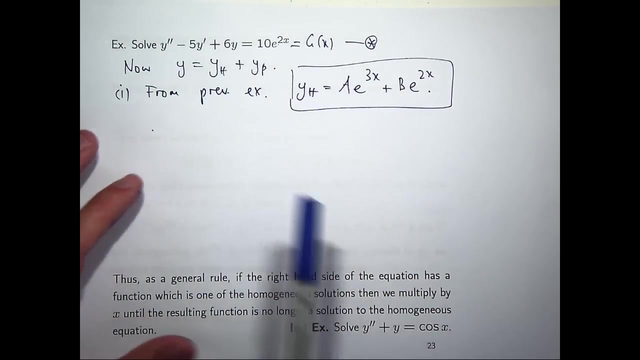 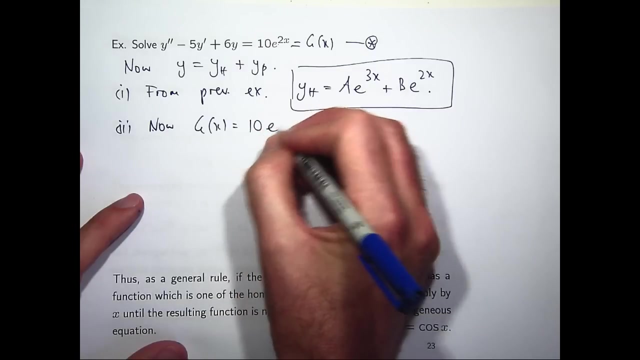 So from the previous exercise, y sub h. okay, So y sub h is something like this: okay, That solves the homogeneous problem. Now, the right-hand side is 10 times e to the 2x. Now what? so? from what we looked at in the previous example, 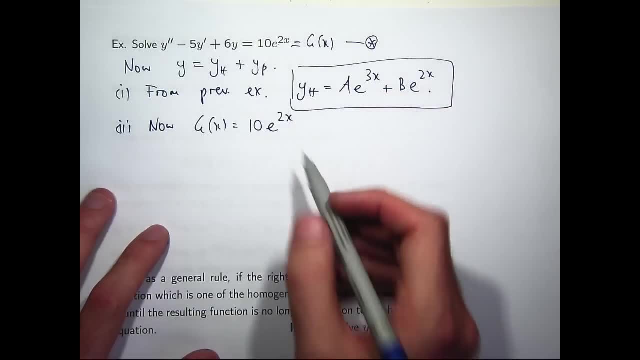 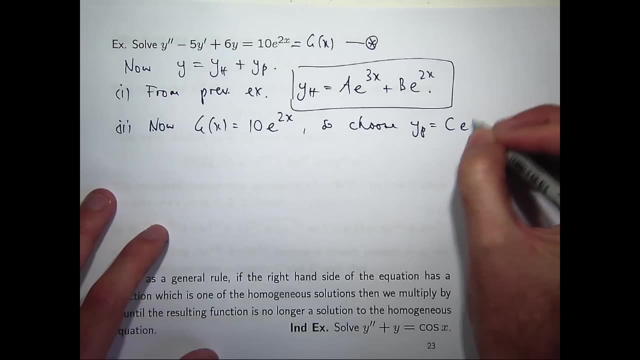 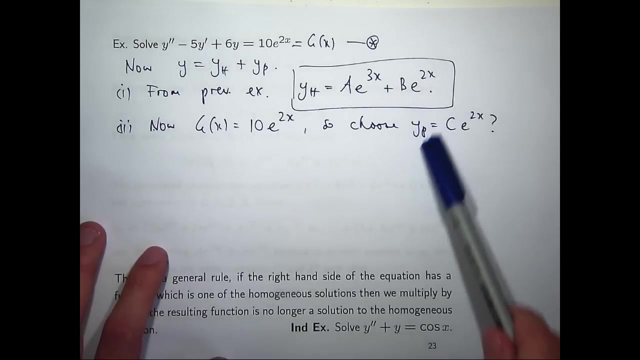 what would you expect a good choice for y sub p to be? Well, It'd be something like this, wouldn't it? If I'm going to construct a particular solution, wouldn't that be a good form? But wait, I'm confused. 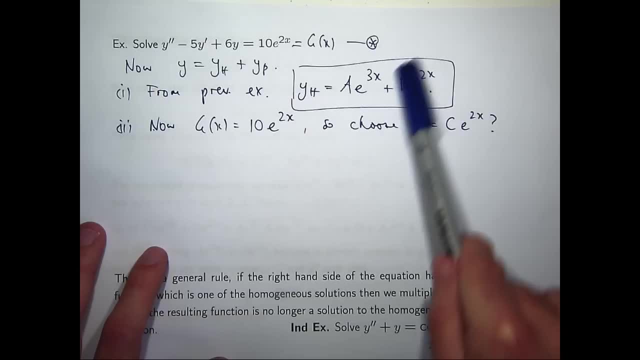 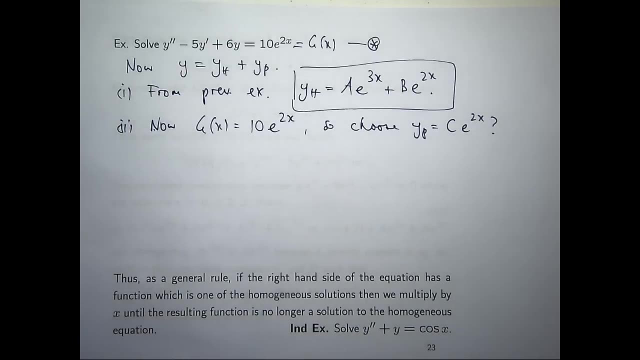 If that is already sort of contained in there. so if I add these two things together, this construction is not bringing anything new. when I add this, I'm going to add them together. okay, Look carefully. The y, sub p, the e to the 2x part. 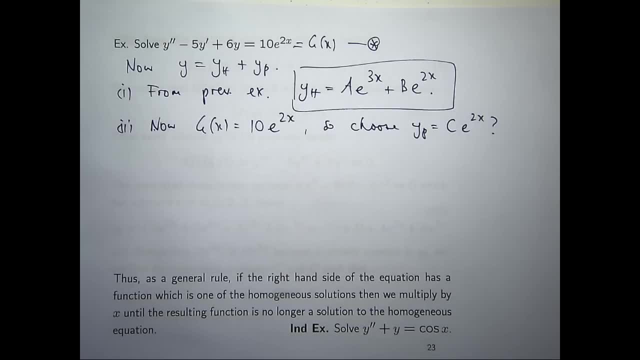 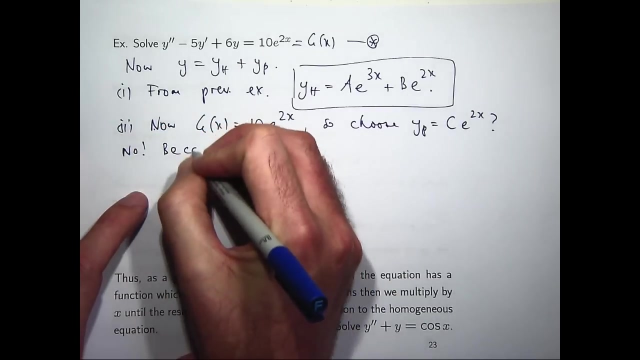 is already contained in y sub h. So if I were to add these two solutions together, y sub p would not be bringing anything new, So this is not a good choice. No, Because y sub p is already contained in y sub h. 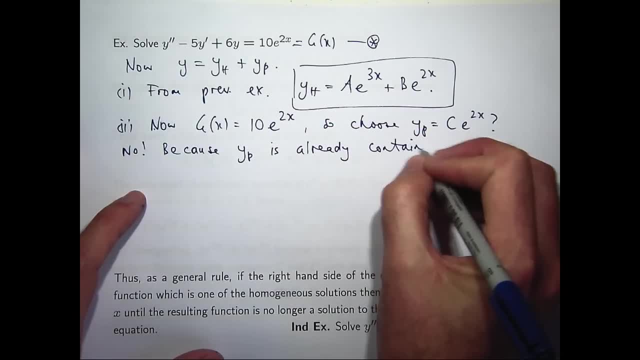 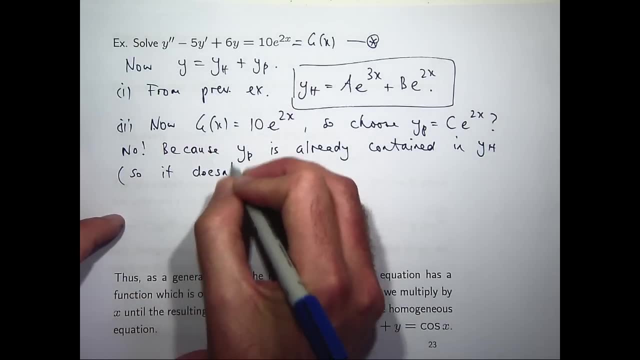 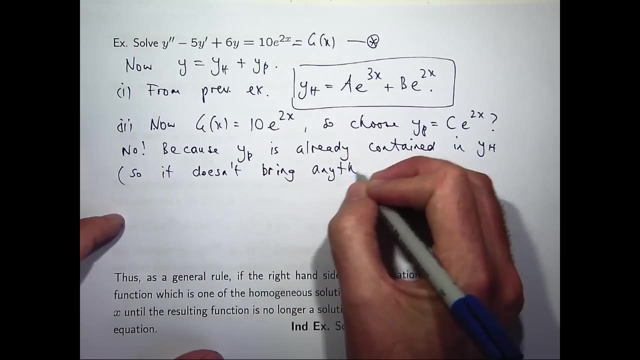 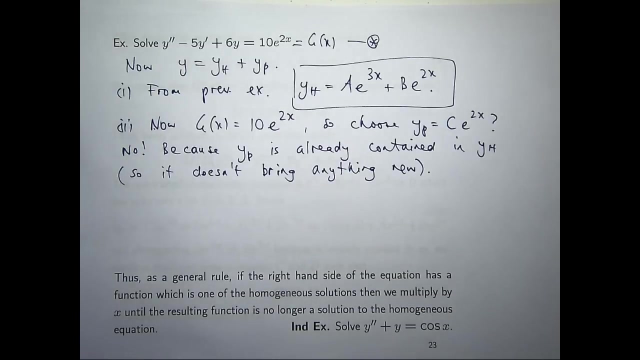 And so it doesn't bring anything new. Okay, so what I'm going to do is multiply that y sub p choice through by x. Okay, So what I'm going to do is multiply that y sub p choice through by y sub h. 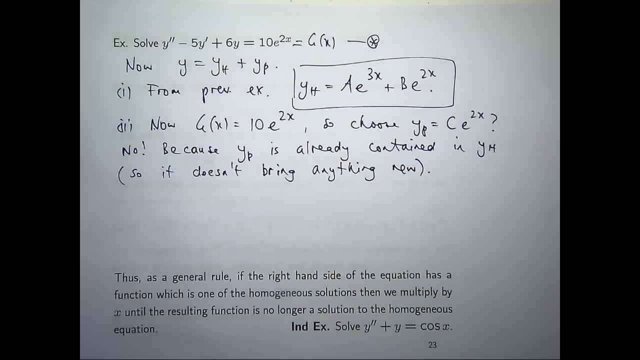 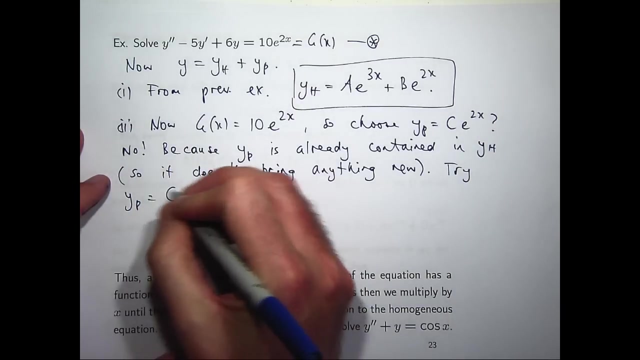 Now we've seen this in a way, when we looked at the homogenous problem with real and repeated roots, We had one exponential plus x times another exponential. So you can kind of think of this as an informal analogue of that. So let's try the following: 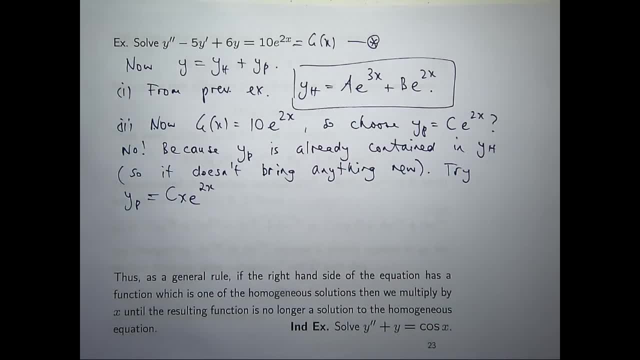 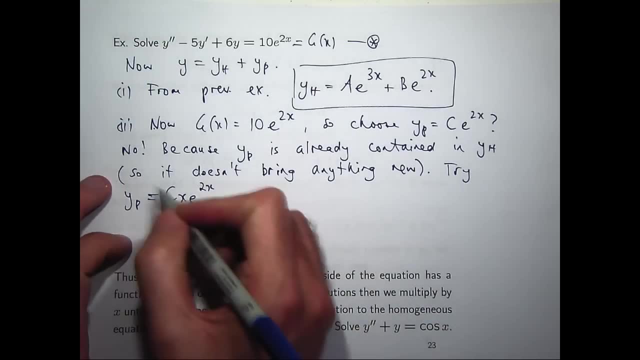 y sub p equals 1.. Mix them up, So 1 plus 1 equal c, x, e to the 2x. Now, Is this contained anywhere in here? Well, no, it's not, Because you've got this x multiplying through. 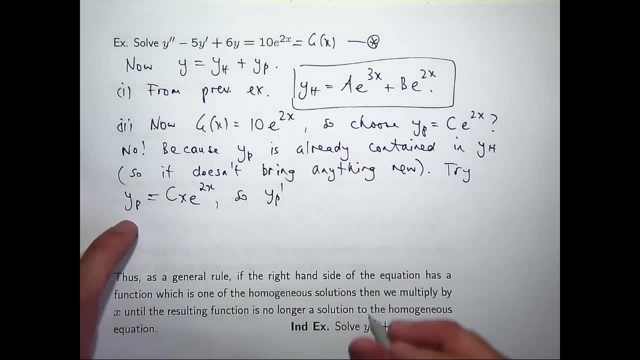 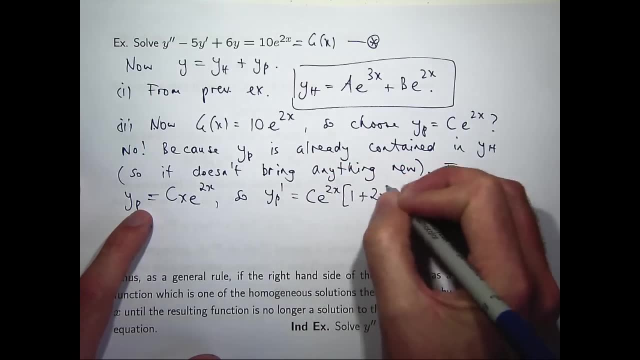 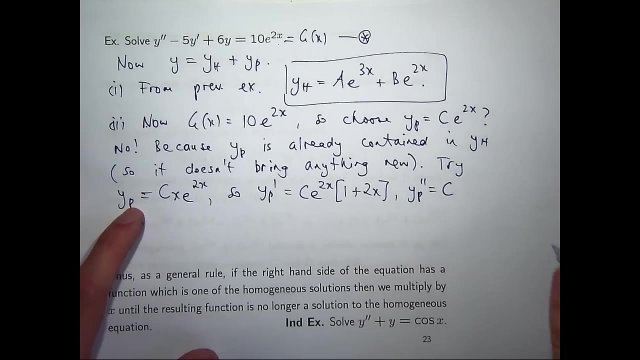 Okay. So let's differentiate this once, differentiate this twice. you need the product rule. So if I differentiate this once, my calculations give me the following: And if I differentiate it twice Again, my calcs give me the following: 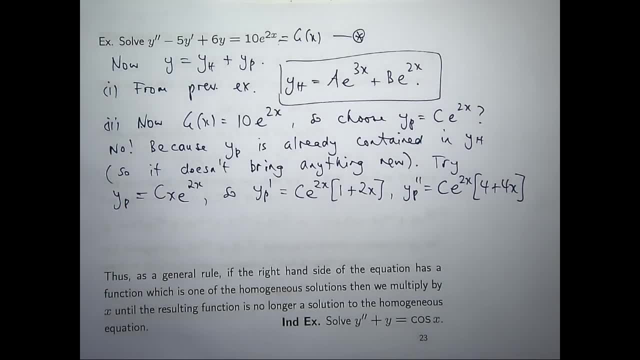 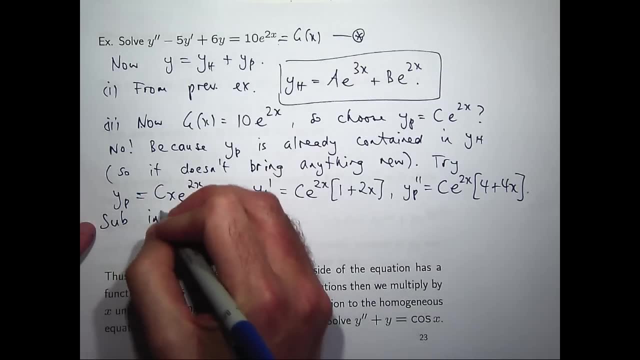 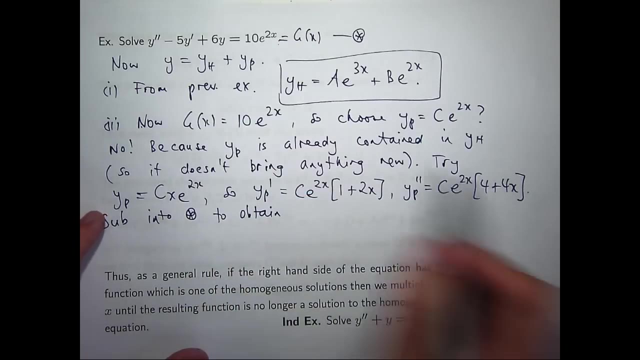 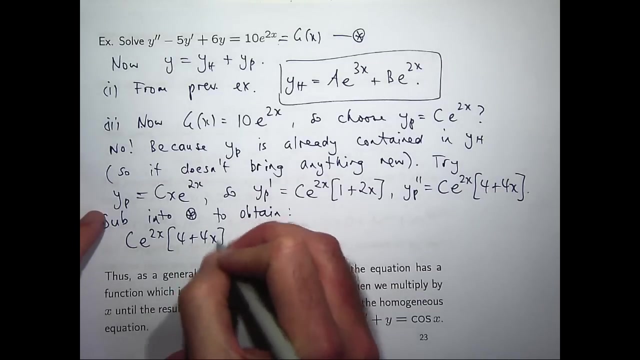 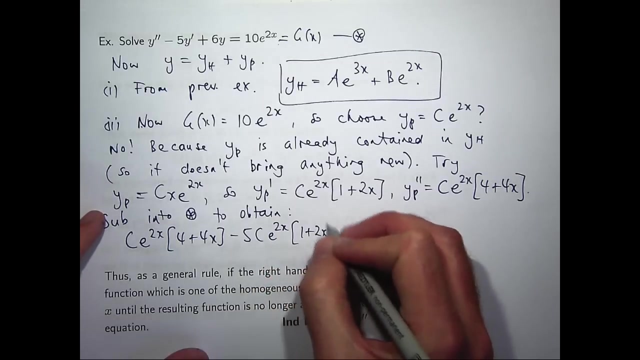 What you want to do is take those three expressions, sub them into star and then compute C. Okay, so we're going to have something like this: C? e to the 2x times 4 plus 4x minus 5 times this plus 6 times. 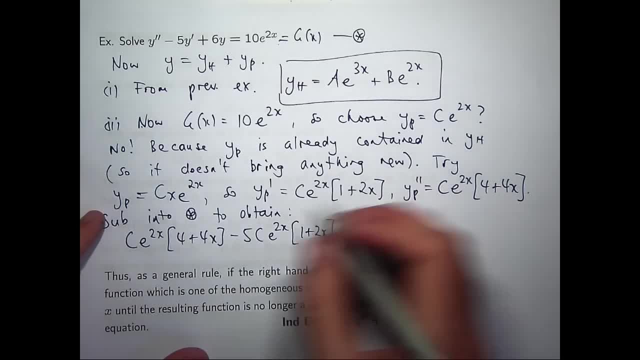 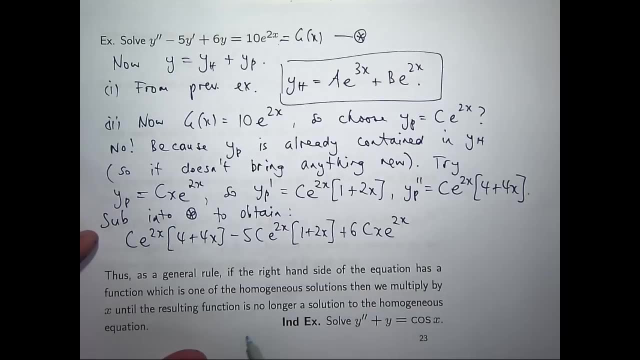 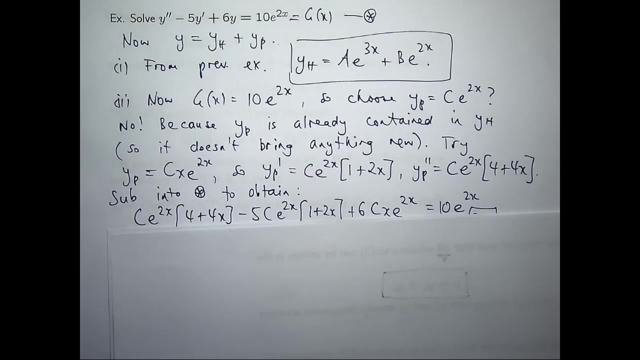 this. Okay, so a little bit of algebra is required, and x times e to the 2x will all cancel out when you expand that. So we're going to get 4c minus 4c. 5c is going to be something like: yeah minus c equals 10,. 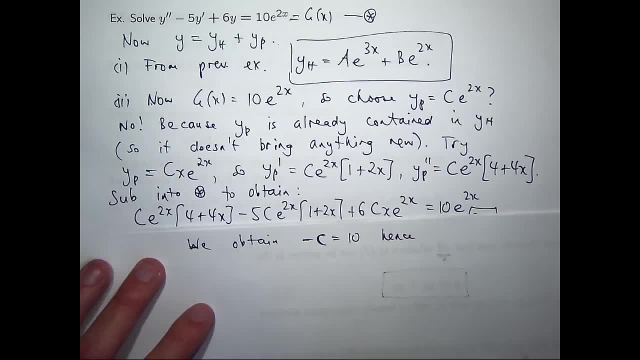 right just by equating the coefficients. So hence this is going to be something like minus 10 e to the 2x. Thus we add our two solutions, Or our two functions, and that's the general solution to our original problem. 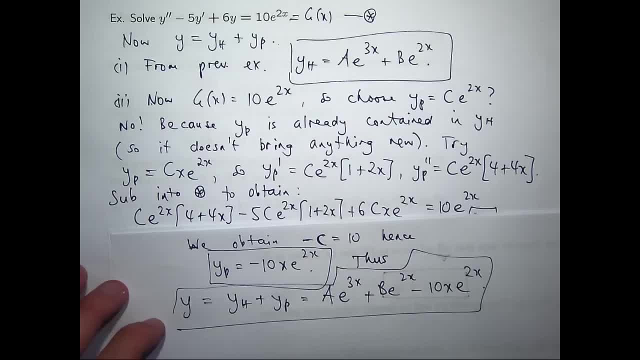 Okay, All right. so the important thing there is: you want to make a assuming you can do the algebra. the important thing is: you want to make a good choice for the function. You want to make sure that, whatever your construction is, it is not contained in this. 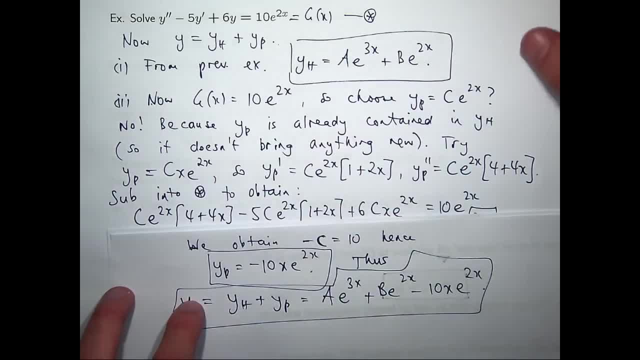 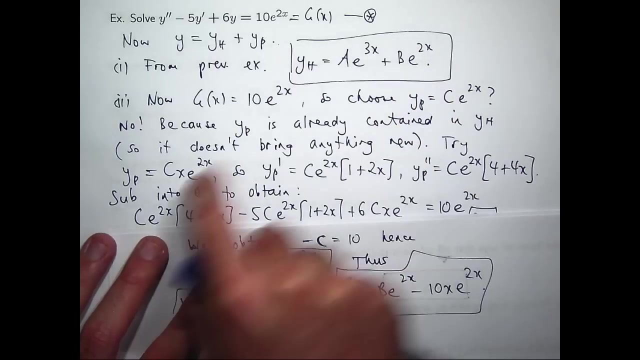 Okay, this is not contained in this. Okay, Oh, good question. Yes, Okay, so that's a very good question. What happens if I tried this and this was already in there? What do you think I would do to this? 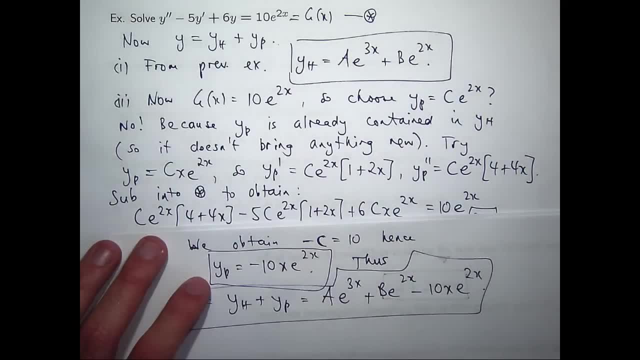 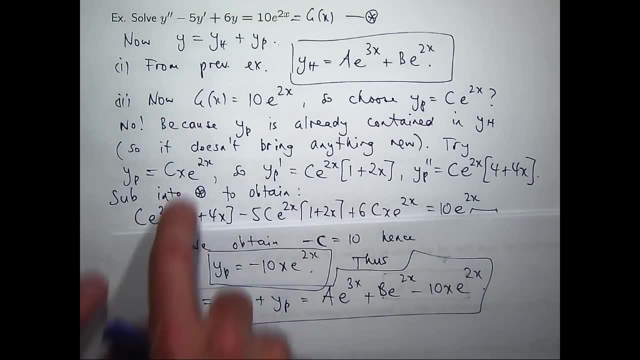 Multiply it by x again, so you'd have an x squared in here. Okay, So I've given you some, so you'd keep multiplying your particular solution through by x or t or whatever the independent variable is, until it's no longer in the homogenous solution. Okay, Okay, So that's a very good question. Okay, So I've given you some so you'd keep multiplying your particular solution through by x or t, or whatever the independent variable is, until it's no longer in the homogeneous solution. 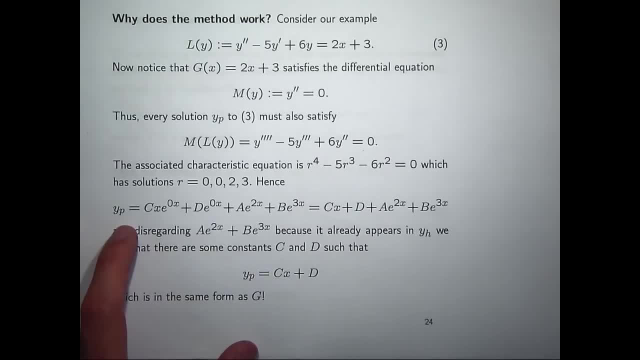 Okay, Okay. Why does the method work When I say that? why can I construct a particular solution just based on the form of g? If g is an exponential, well, I'll just make my construction an exponential Well. that's a very good question. 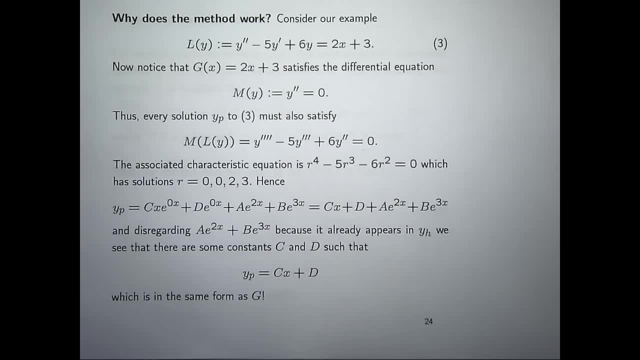 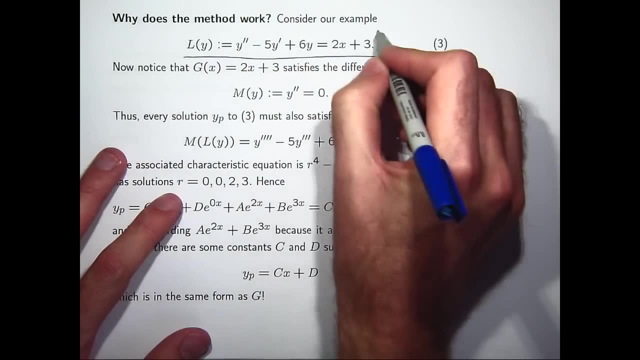 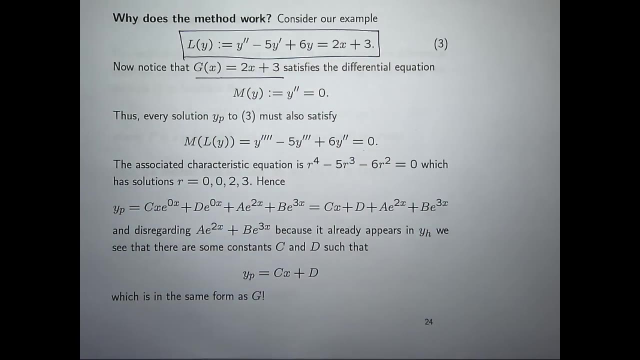 Some of you may know how to do this process, but why does it work? Okay, This is the original example that we looked at. The right-hand side is like a linear-type function. What we do is suppose y sub p is a solution to this. 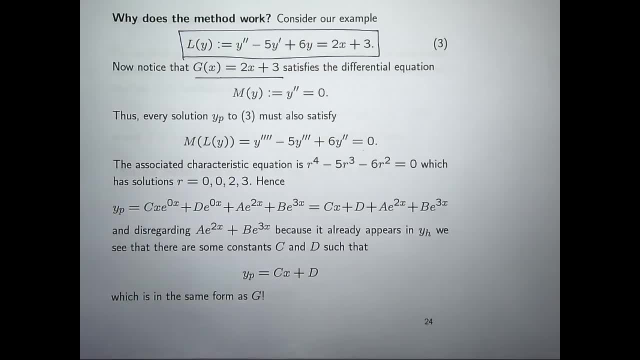 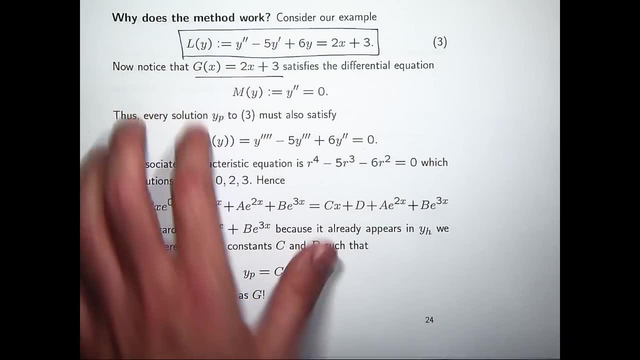 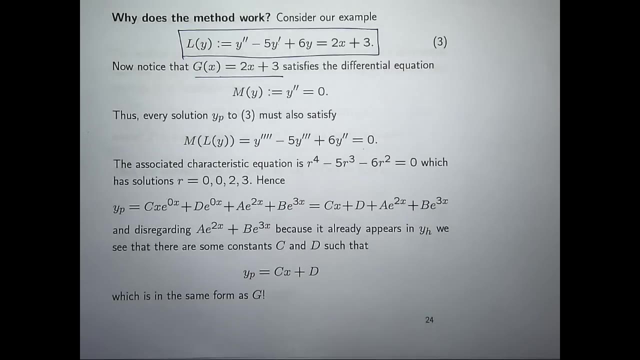 We don't know what it is, but let's just try to construct it. What I can do is differentiate the original ODE in some way that annihilates the right-hand side. Okay, If you look closely, 2x plus 3, if you differentiate that twice, it gets annihilated to zero. 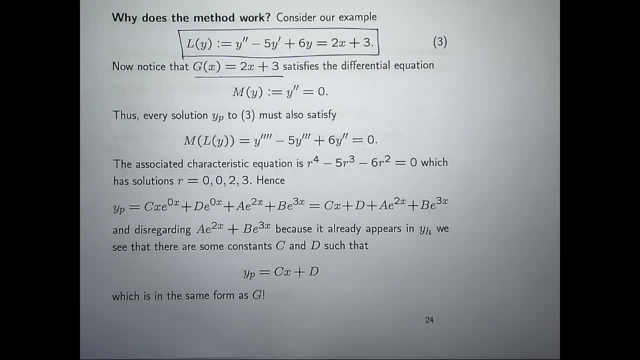 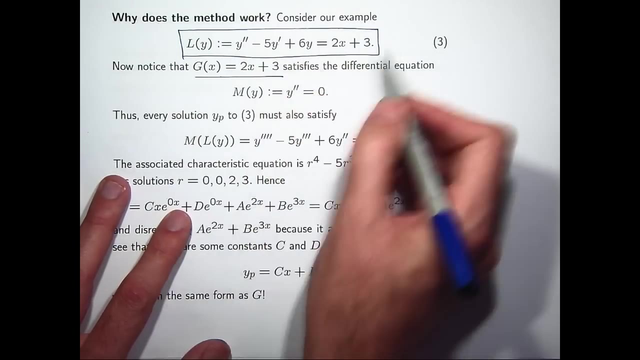 It disappears. So what I can do is introduce a new linear-type operator, m, just in this case defined by this, And if I take, basically if I differentiate twice both sides of the equation, I'll get this particular problem. 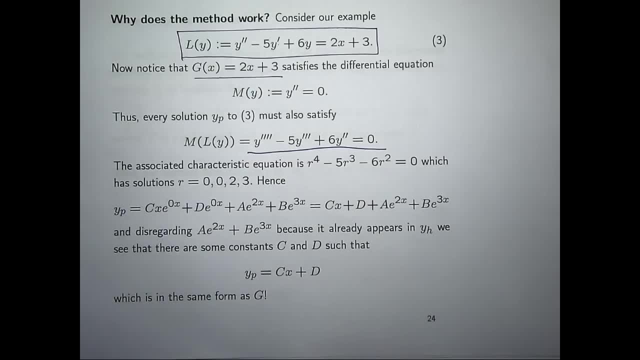 Now this particular problem. it's a higher-order problem, fourth order, It's linear and it's got constant coefficients. Now we can solve that just by the methods that we already know. The only difference is our characteristic equation is going to have a higher degree. 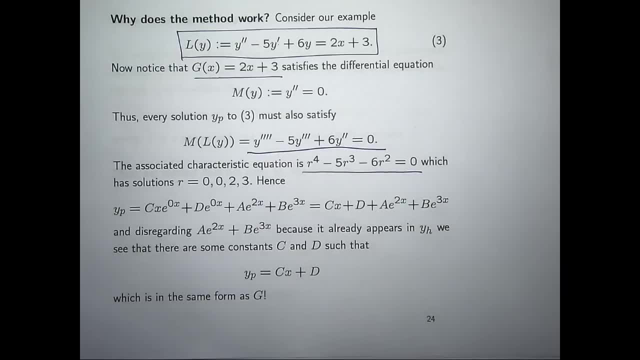 It's going to involve something like r to the power 4. Solve the characteristic equation. you get the following roots: You get zero as a repeated root, positive 2 and positive 3.. So the basic theory says that a solution to this homogeneous problem will be something like this: 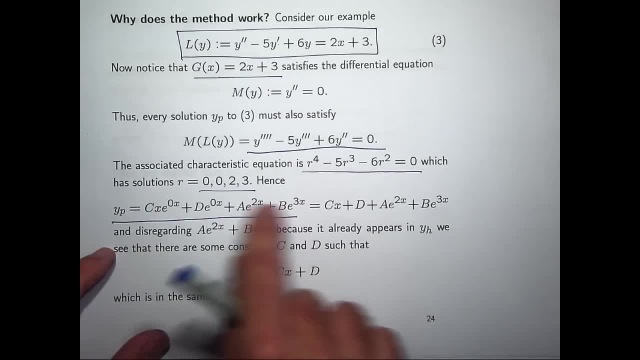 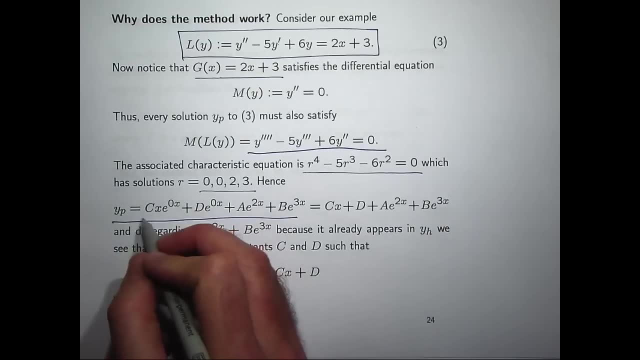 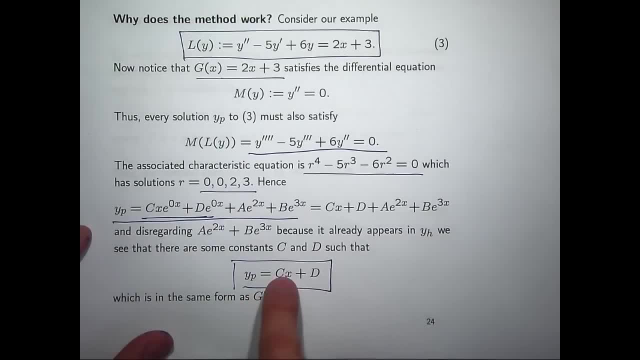 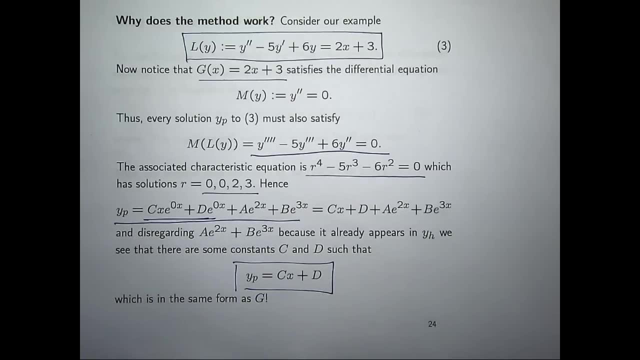 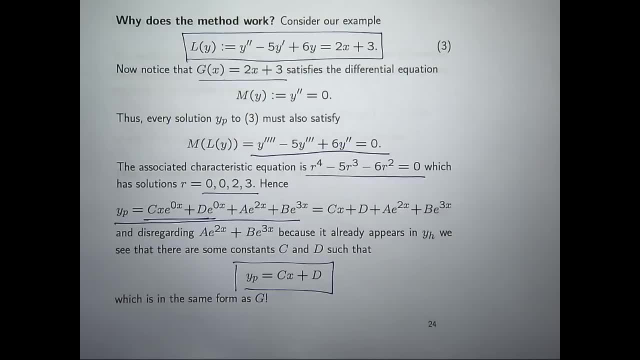 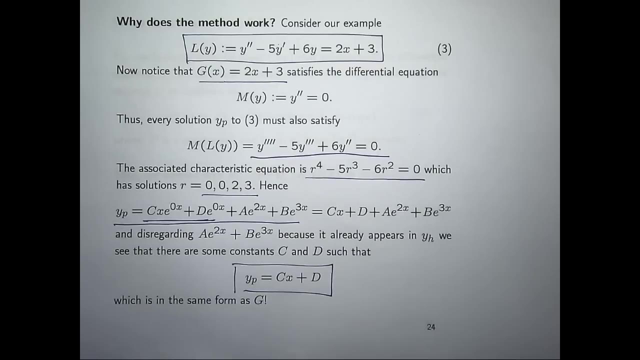 such that you can assume a particular solution. has that Cx plus d form? Okay, Very powerful method known as the annihilator method. Okay, You annihilate the right-hand side until it disappears. Now, the choice of annihilating operator here, the choice here, is dependent on this. 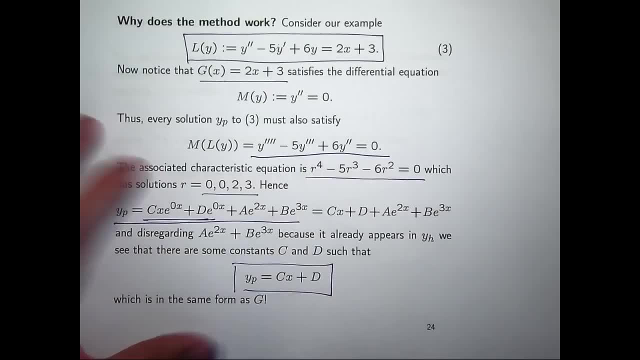 So if this was e to the x, you would choose: m of y equals y prime minus y, Because you know y prime minus y. if I, you know e to the x satisfies that Okay. So this is why the method of undetermined coefficients only works. 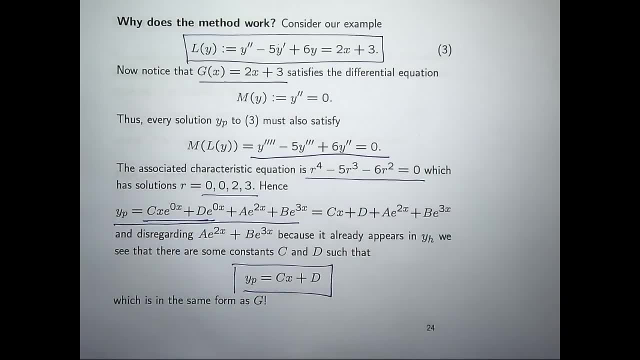 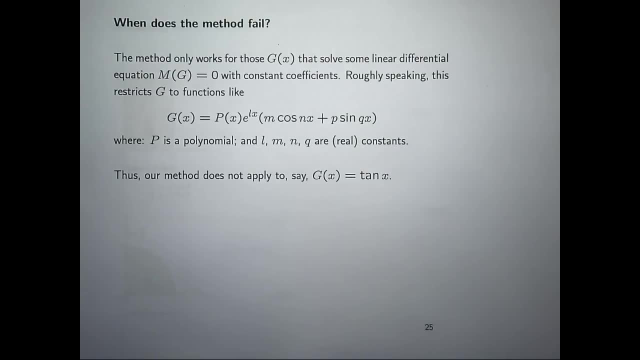 with certain kinds of functions on the right-hand side. You can't annihilate all of them. You can't annihilate all functions, okay, through differentiation. Okay, Think of tan x. How would you annihilate tan x through differentiation? You can't. 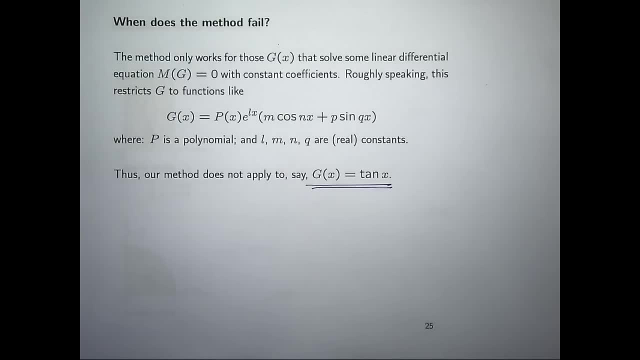 You can't do it Okay. So this is why we say our right-hand side's. It means that when we say that, it means that we can annihilate it through through some sort of linear differential operator with constant coefficients.